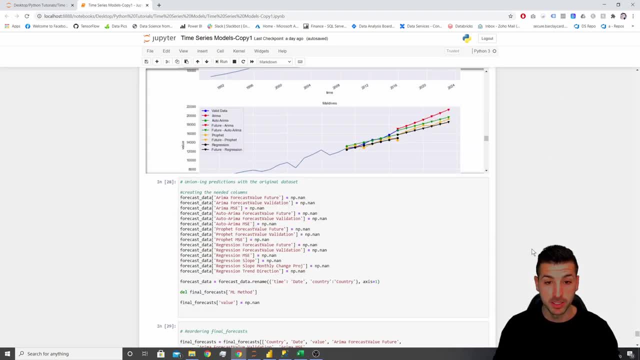 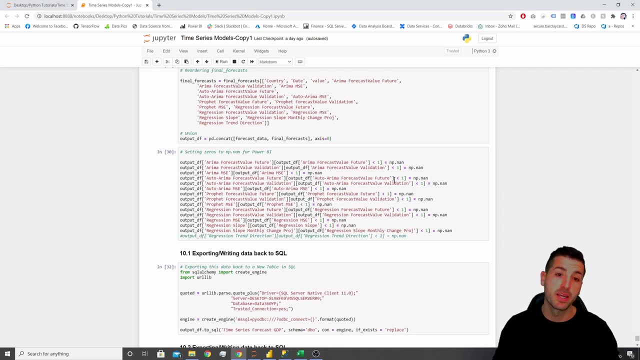 which is about 230 countries in our dataset Then. so this is all the output from all the countries, and at the end I'm going to show you how to combine the actual data with the forecast, and then we're going to export the data both in. 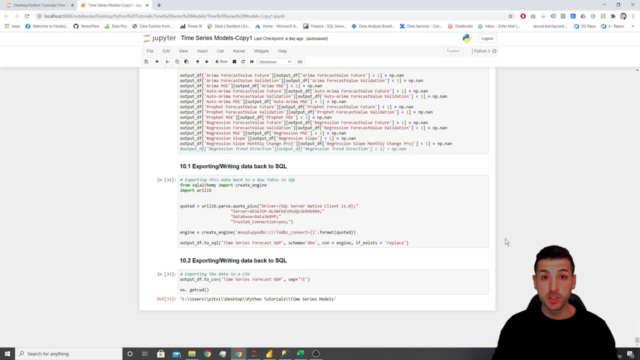 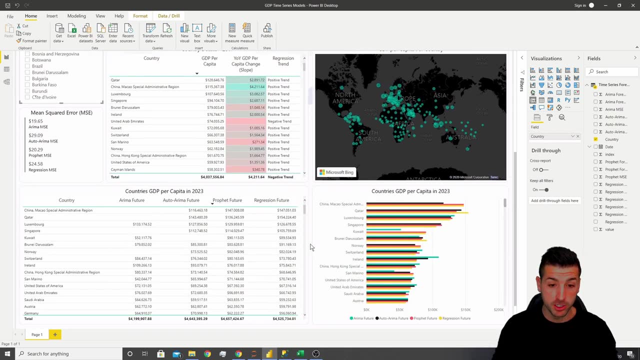 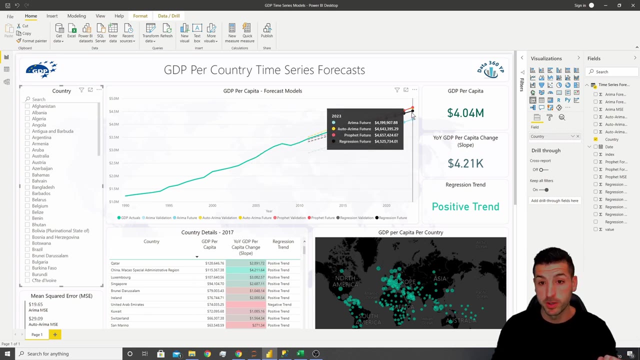 a csv and in an sql database. Afterwards I'm going to show you how to take your results and predictions and build this Power BI dashboard from scratch. Here we can see all the countries, there are actuals, there are validation predictions and there are future predictions. 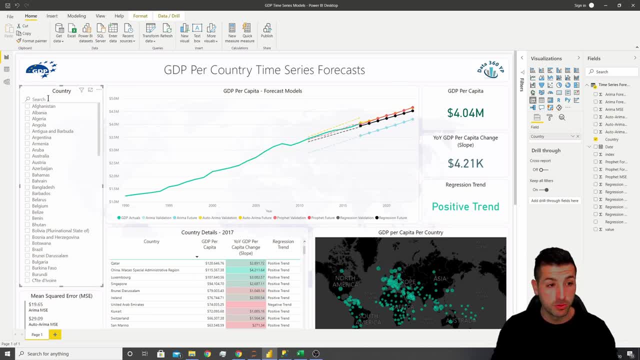 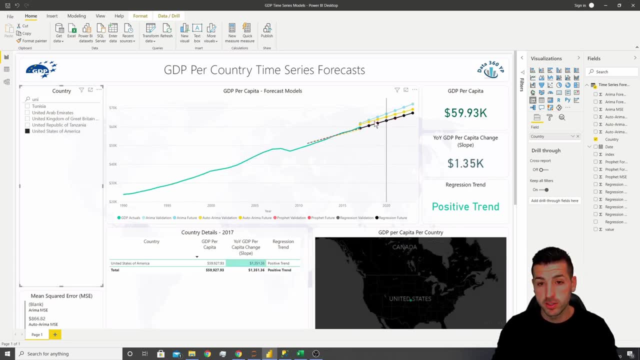 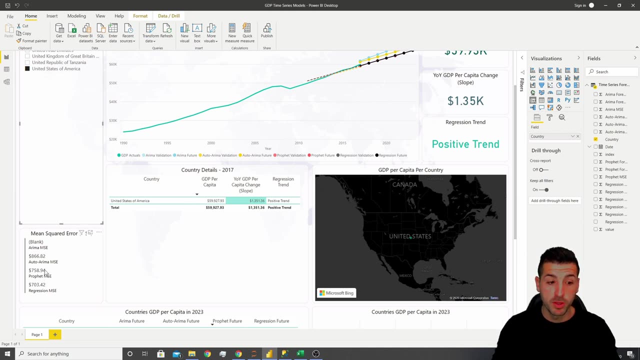 all the way to 2023. and if we were to select a country, for example, so let's do United States of America. we can see the four models and their predictions. we can see the mean square error. so if we were to choose the best model, it was going to be the one with the least mean square error. 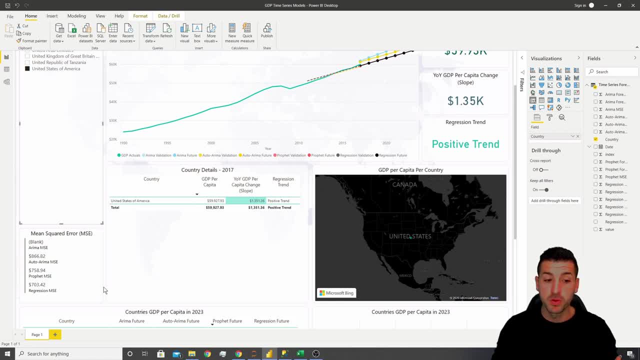 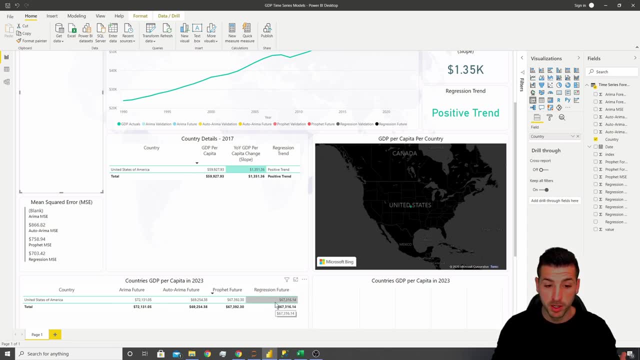 so that was going to be the regression mean square error. so if I was to do a prediction for the United States, I was going to choose this number over here for 2023.. I have all four models here and we should expect the GDP per capita of the United States to be about: 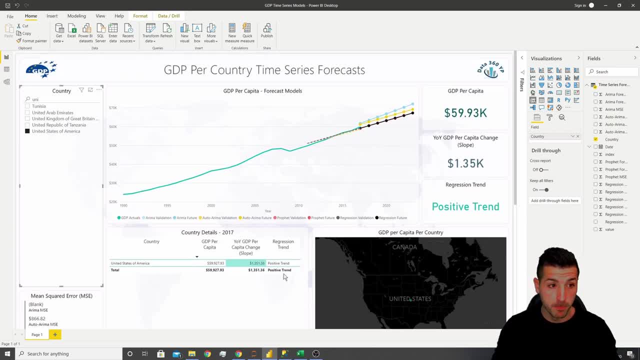 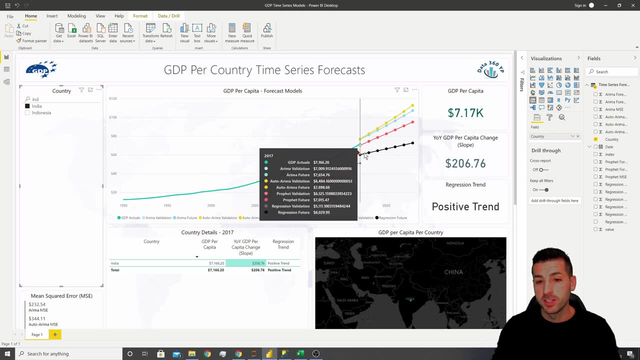 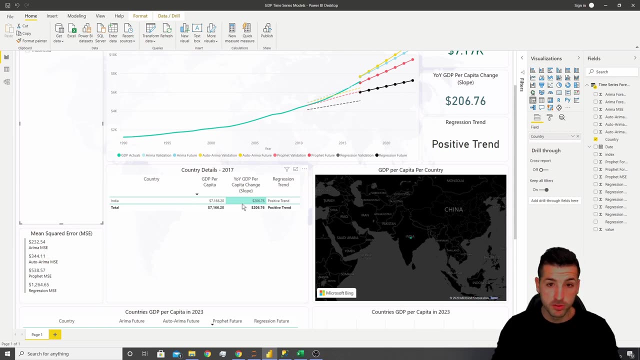 67,000 for 2023.. We can do this for any country or all countries together. so if we check India, for example, we can see there is a bit of difference in the models, but we can choose the one with the least mean square error, which is the ARIMA one. so that's going to be the green one. 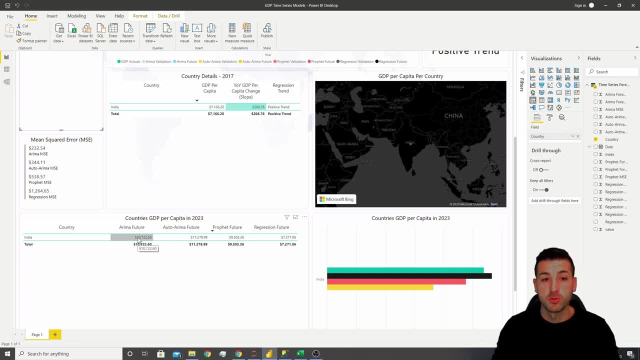 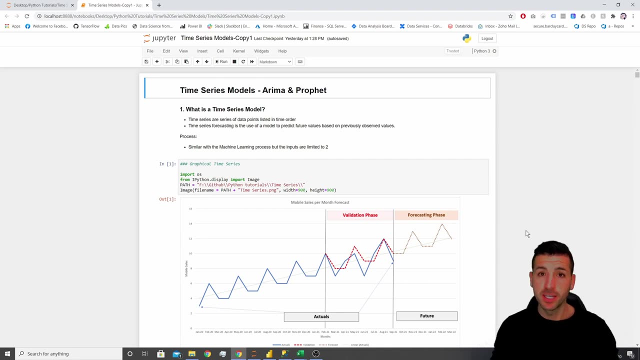 so that's going to be this one over here. so we should expect an increase from 7,000 into 10,000 GDP per capita for India in 2023. right, and before we start this tutorial, if you're new to my channel and you're passionate about data science, please consider. 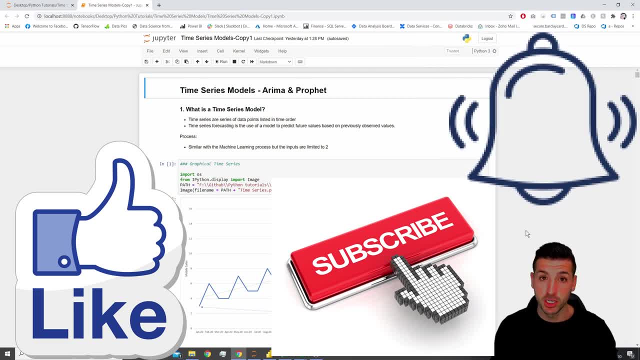 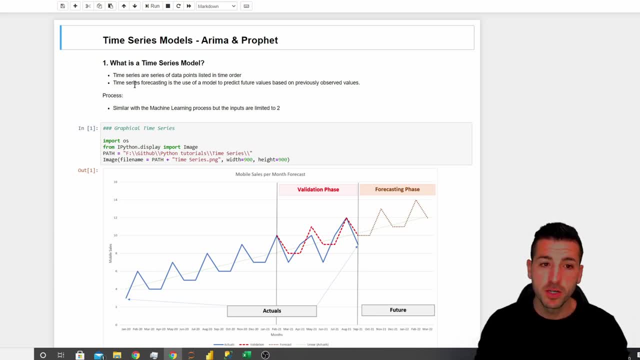 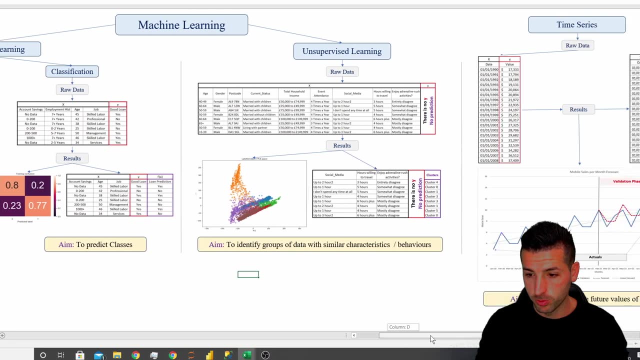 liking this video, subscribing to my channel and enabling notifications for my future videos. right, so let's start. what is a time series model? the time series are series of data points listed in time order. so if we go over here just to show you an example, time series is when we have a series of 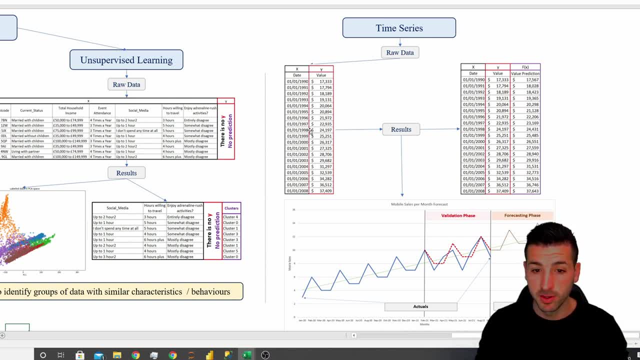 dates. so you can see here it starts from 1990 all the way to 2008 and we have some values. then we take these raw data, we feed it into a model and we get a value prediction for each date or we can forecast going forward. so if I go back again, time series forecasting: 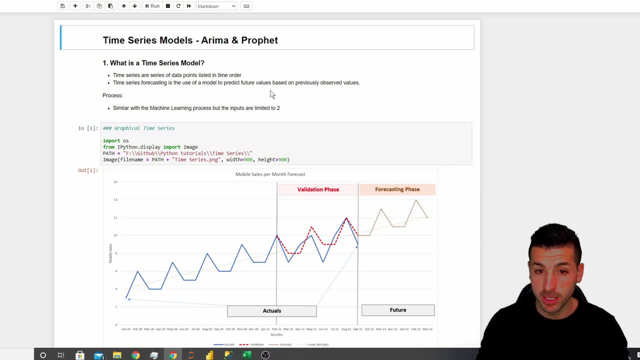 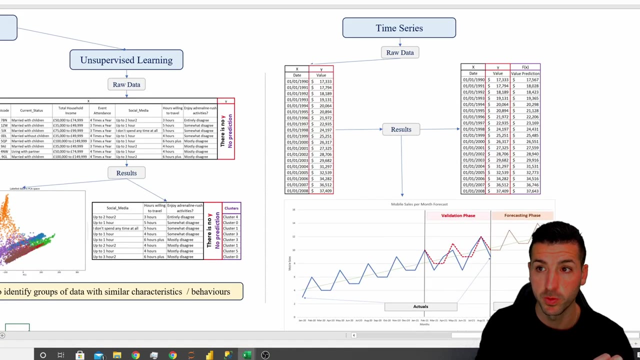 is the use of a model to predict future values based on previous observed values. and then the process is similar with the machine learning process, but the inputs are limited to two inputs, as we have shown here. we only have date and value and we predict going forward. so if we go through the machine learning process quickly, we start with the problem. 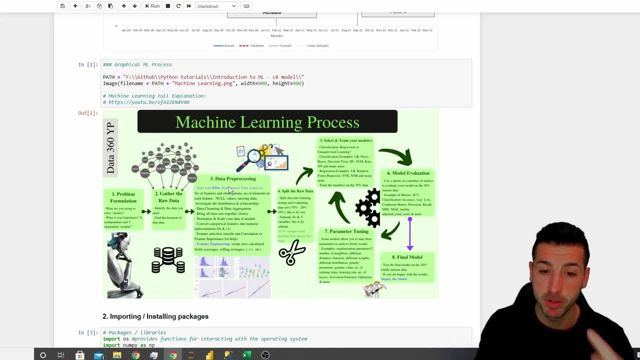 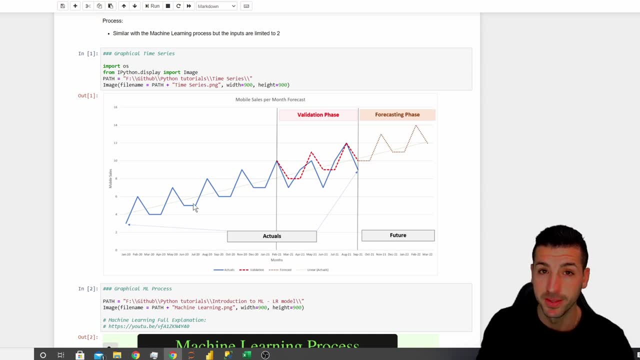 formulation: we gather the raw data, then we do our data pre-processing and then we have to split the raw data. so this is where we take the split. as you can see in this example, we have the mobile sales per month and year. so we split the data somewhere around here, then we select and train. 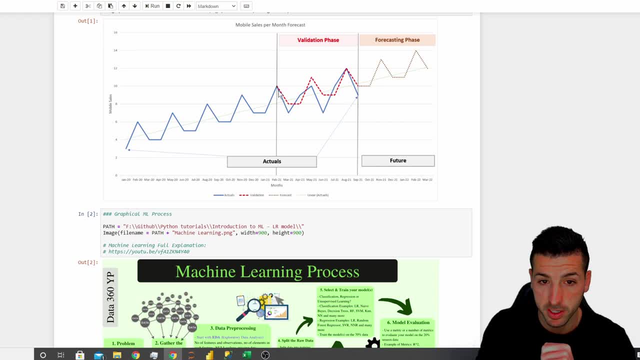 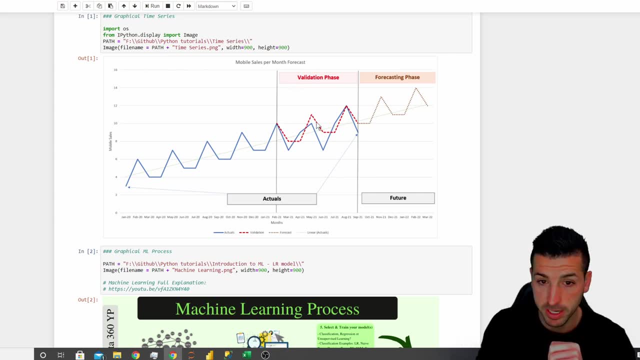 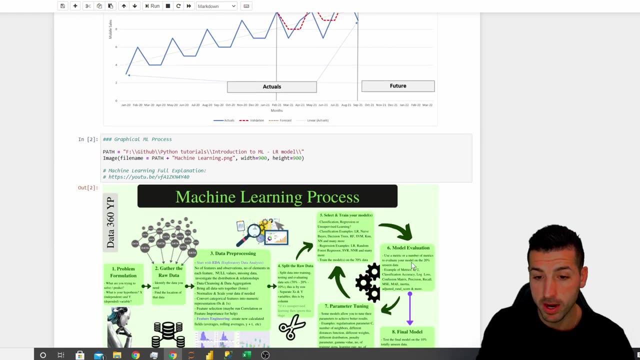 our model based on these data. so these are x train all the way until here. then we do the model evaluation, so we predict which is the red dotted line and then based on a metric, so we're we're going to use mean square error, We are going to evaluate our model and then we are going to do. 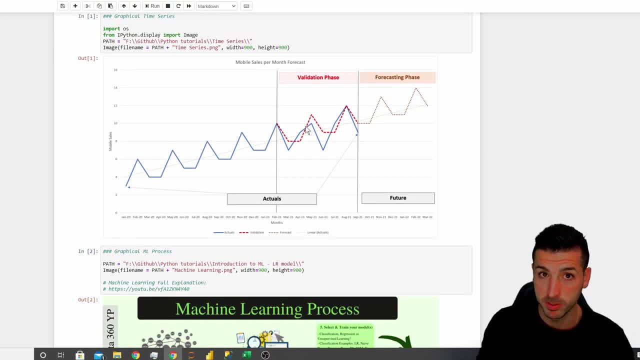 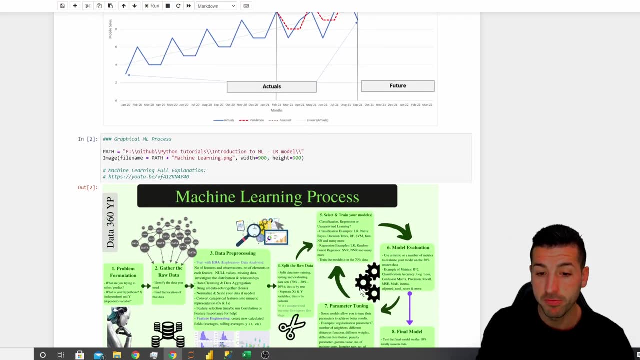 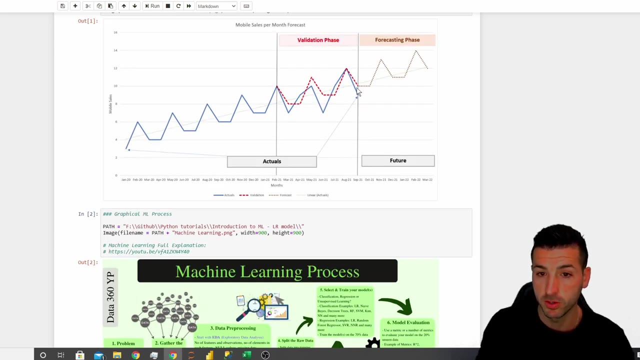 parameter tuning. So we are going to adjust some of the parameters so we can minimize the mean square error as much as possible and improve our model. After we are happy with our model, we are going to run our final model. So we're going to use all the data from here to September. 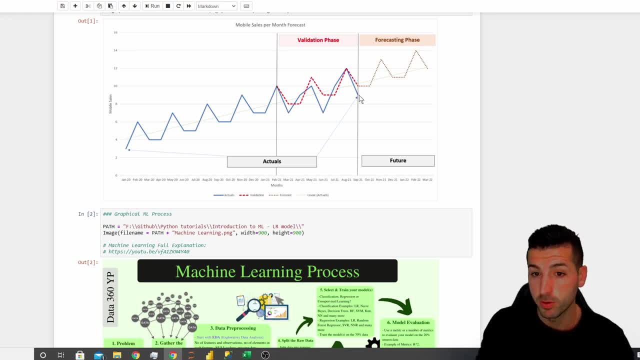 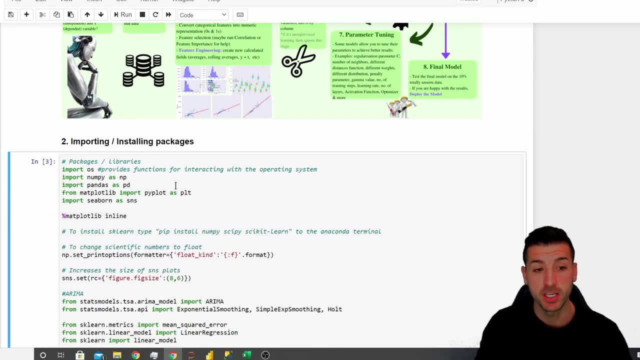 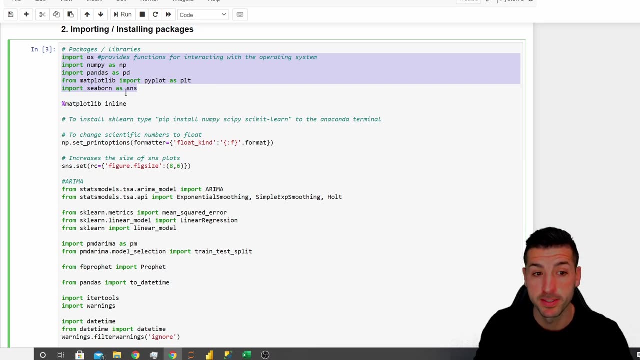 2021 to train the model and then run a forecast on the future, which is going to be this dotted line over here Right moving on. we have our packages and libraries, so we're going to be using all the main ones. so operating system, numpy, pandas, matplotlib and Seaborn Additionally. 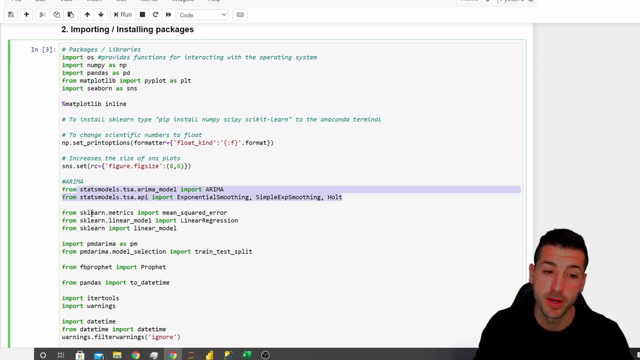 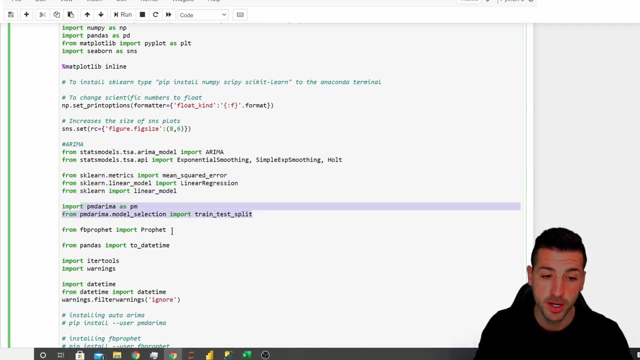 we're going to be using from stats model, the Arima one, from sklearn, the linear regression libraries. These libraries are for the AutoArima- This is a for profit- and some additional libraries for daytime. so if you're missing any of these libraries, 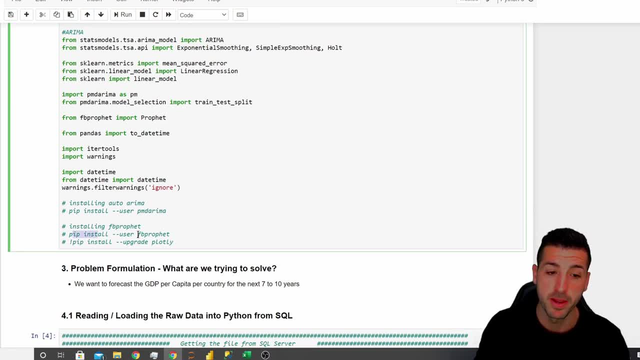 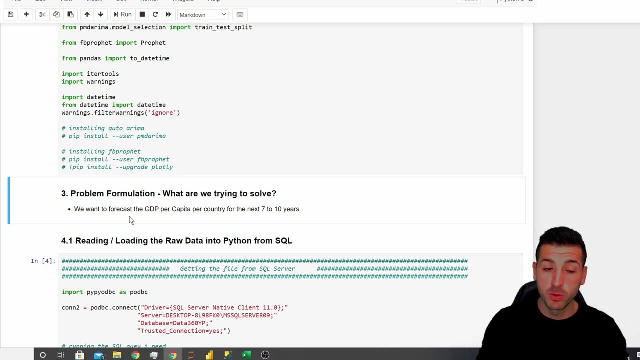 or packages you can run: pip, install and then the name of the library and that's going to install it on your pc. right moving on is the problem formulation phase. so here we need to ask the question of what we are trying to solve, and the answer is that we want to forecast the gdp per. 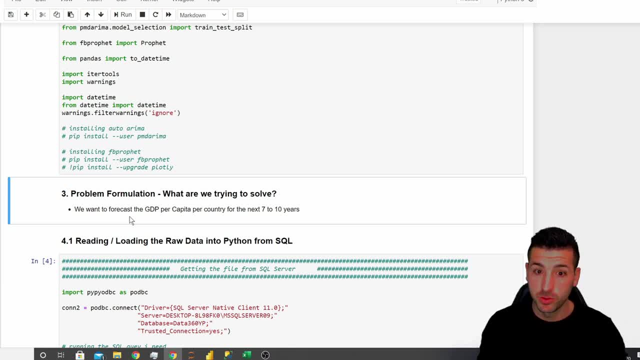 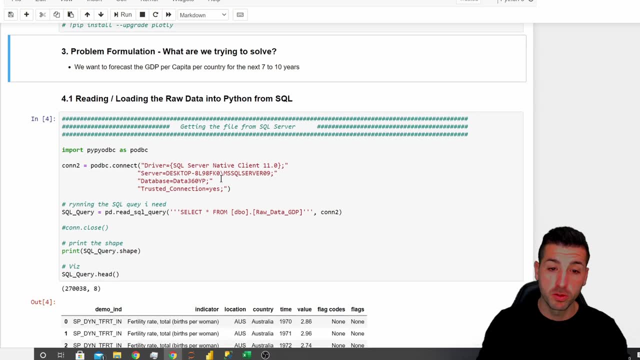 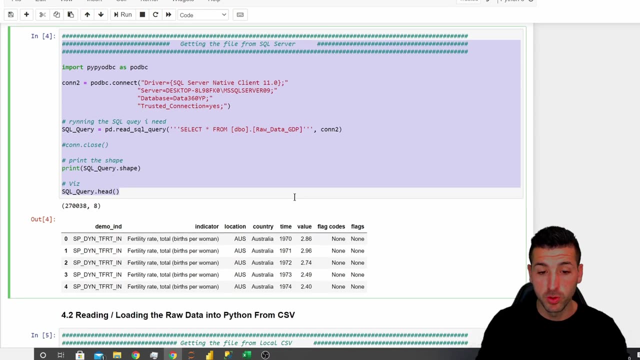 capita per country for the next seven to ten years. so that's what our time series models are going to be forecast. moving on, we need to load our raw data. so here i load the raw data from an sql server. but for you, i'm gonna be providing you a csv file where you can load the raw data from a csv file. 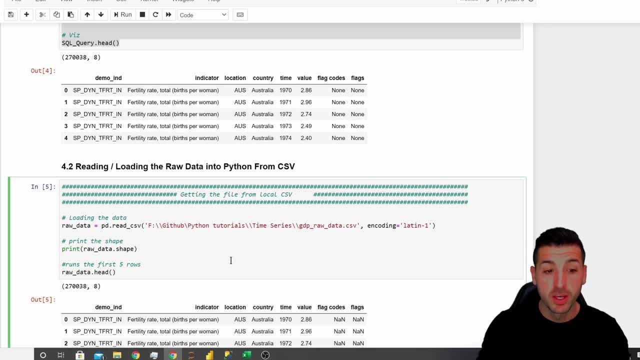 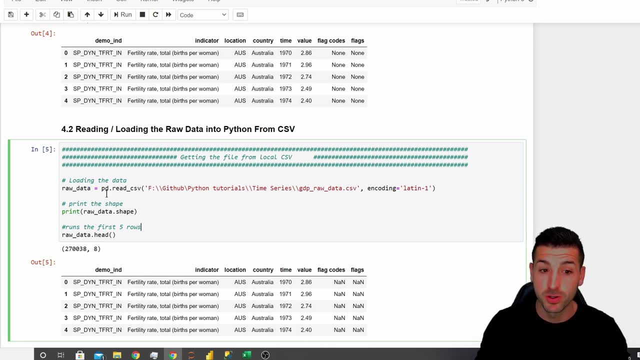 so i'm gonna have the links in the video description below in order to load the raw data. now all you have to do is set up the gdp per country and then set up the gdp per country. row. data equals pd. dot. read underscore csv. then in here you're going to need to paste the path. 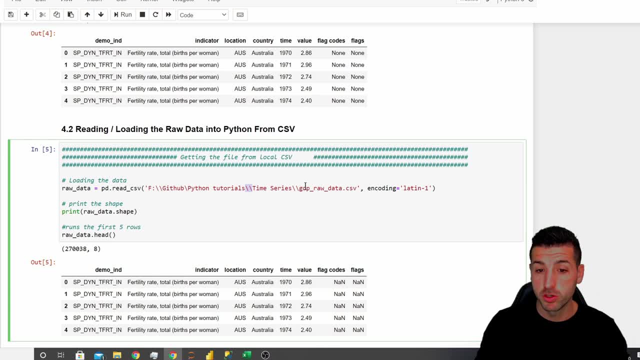 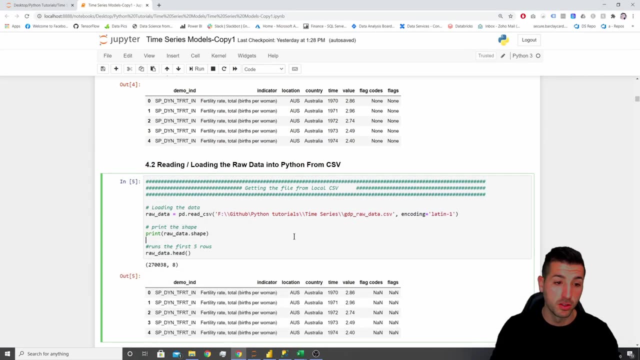 where you have downloaded the row data and also at the end add the name of the file and a dot csv. also use encoding as latin slash one, and this is going to load the row data from excel, so this row data is going to load it into row data over here. then what i do here is that i print the shape. 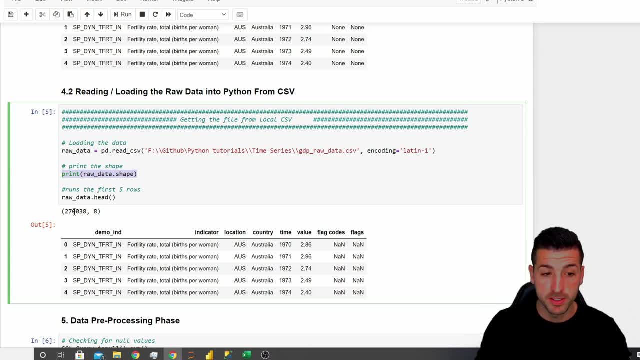 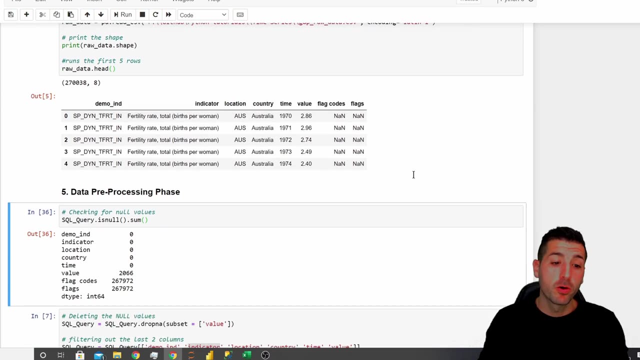 of our data. so our shape is 270 000 observations and eight columns, and i also print the head of our data frame so you can see we have all the columns and the first five rows of our dataset right next we need to go through the data pre-processing phase. so the first thing i always do is check for. 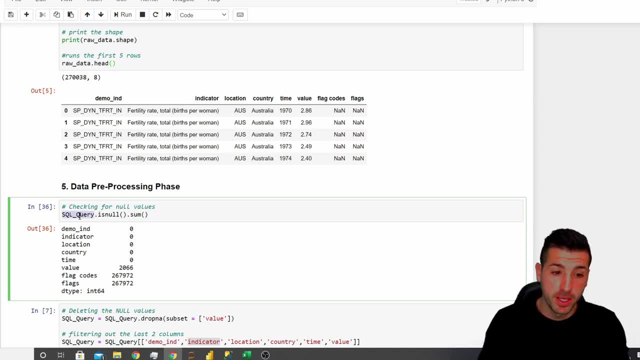 null values. so by adding our data frame here and then saying dot is null, dot sum, we're going to see the number of columns that we need to print. so we're going to print the first column we need to of rows that have null values. By the way, I'm not using this row data. 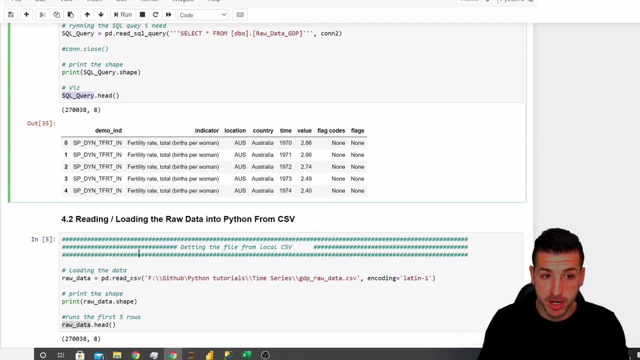 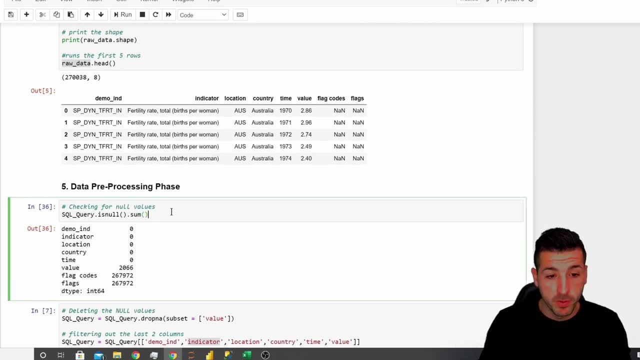 I am using the SQL row data, but both of them are the same. One of them comes from SQL, The other one comes from a CSV is exactly the same data frame. Anyway, as you can see, we have about 2066 null values in value. 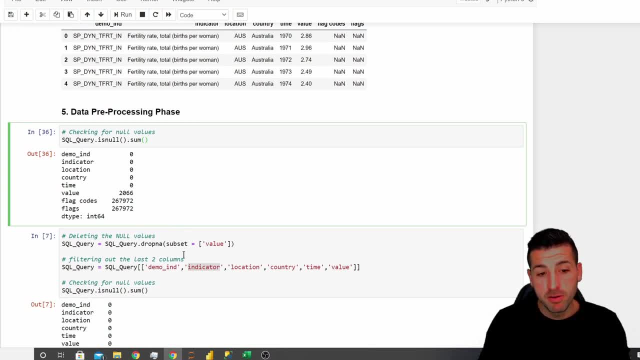 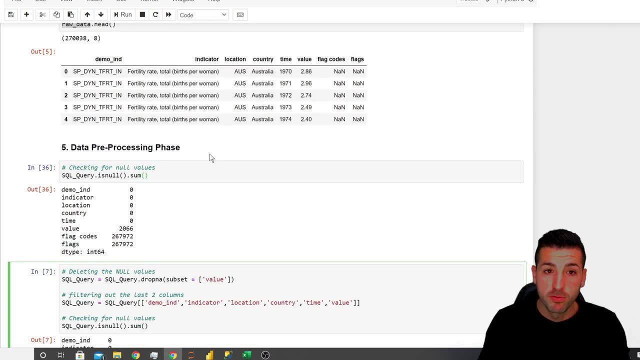 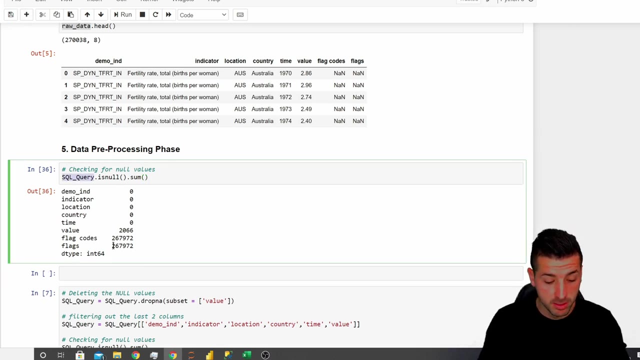 So in here. so we need to investigate this. However, what I did is that I went straight for the delete, because I know that these null values do not come from the GDP per capita indicator that we are going to use. And just to show you how to investigate this. 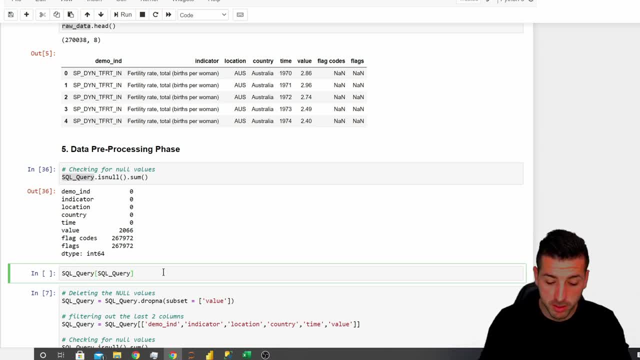 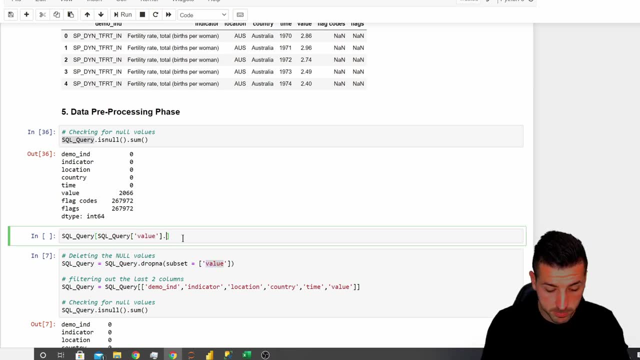 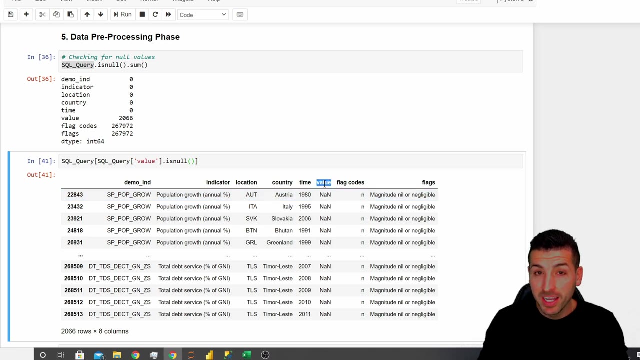 investigate the nulls we can do. we can write this query So we can add the value and then say dot is null. So this is going to return all the rows that have a null value in value. However, I only want to investigate the indicators. 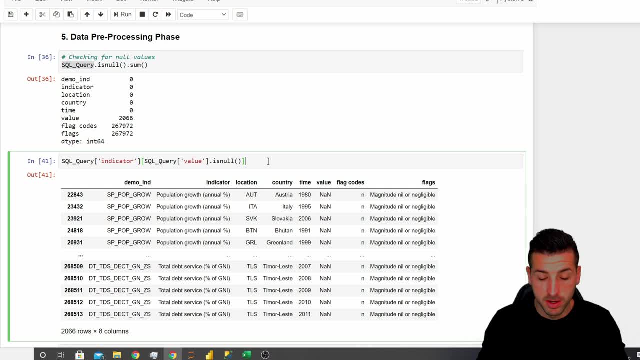 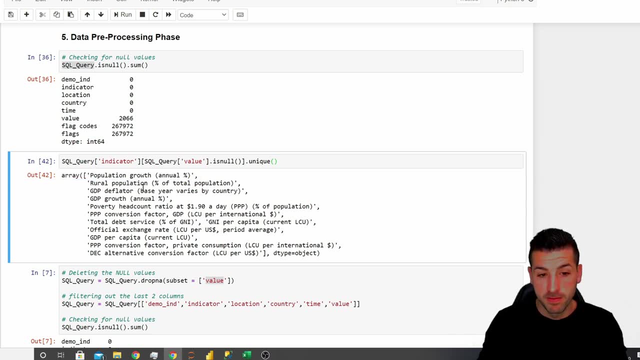 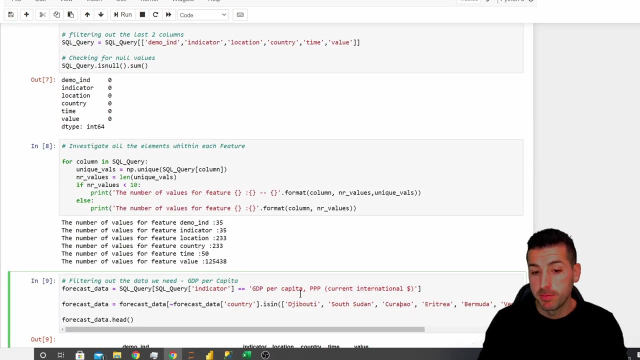 So if I add the indicator in here and then I'll say dot unique, we can see that unique indicators that have null values and the GDP per capita, which is this one over here, GDP per capita comma PPP- current international dollar- doesn't have any null values here. 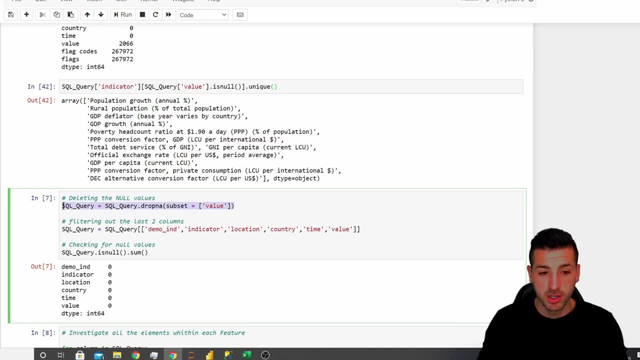 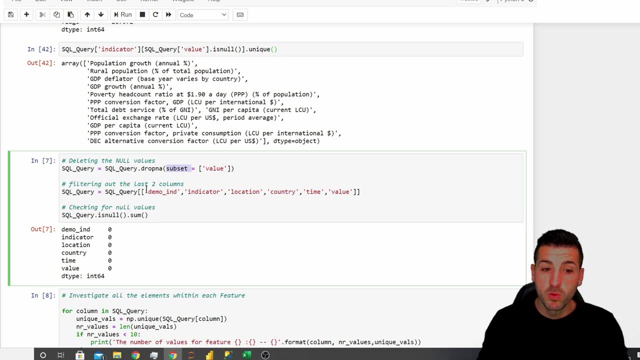 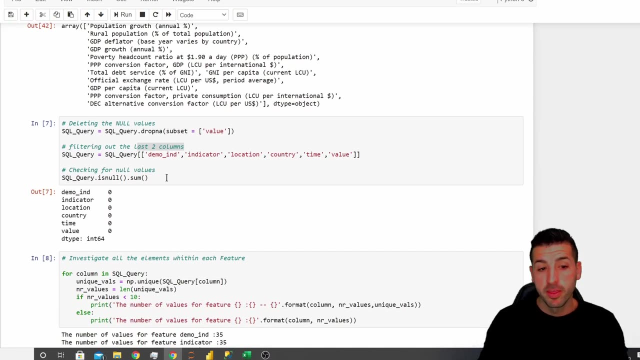 And this is why I drop the null values straight away. as you can see, sqldropna from the subset of values and then I'm also removing the last two columns, so these two columns that are full of null values and I don't need. Then I check again for null values and I don't have any null values. The next thing I do 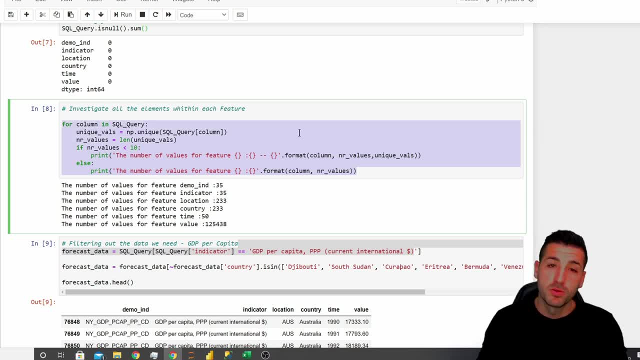 is a standard piece of code that I always run to investigate all the elements within each feature, and what this code does is that it goes through every single column from our data frame and it prints out two things: Either the number of distinct values- so 35 distinct values- or the 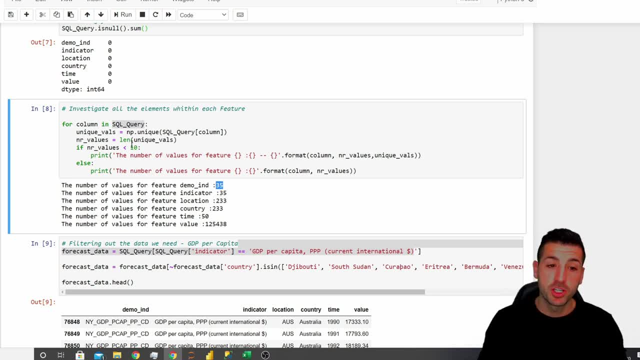 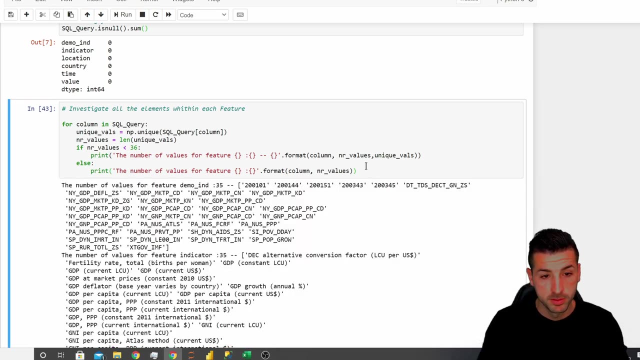 actual elements within the column. So if I change this number of values to, let's say, more than 36, so it's going to pass the threshold, It's going to print all the demo ids and all the indicators. So if I run it again, you can see. now it says the number of values for. 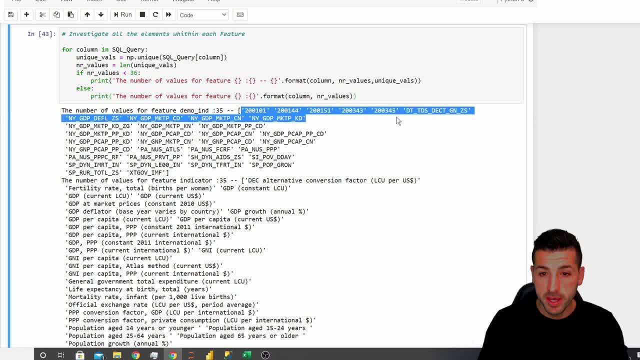 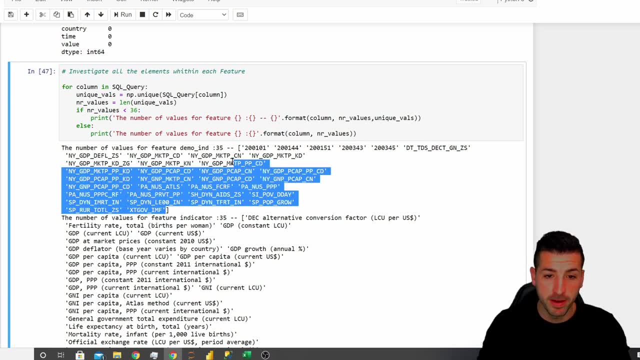 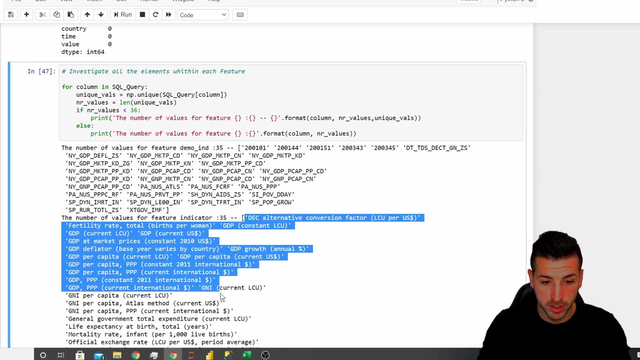 feature demo int is 35, and then it prints all the 35. So one, two, three, four, all the way to 35 distinct demo ids. and then it does the same for the indicator. So it prints all the 35 indicators up until here. So these are all the indicators. 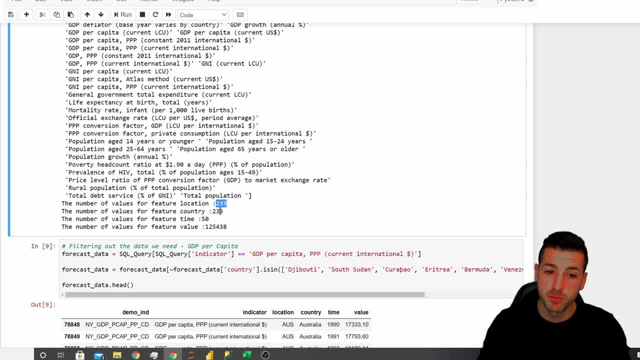 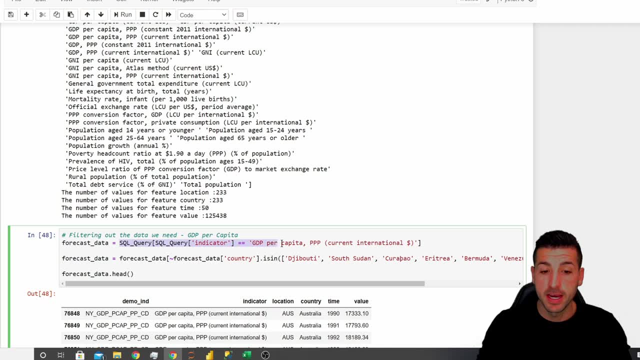 And then for the location, country, time and value, it just prints the number of distinct values in those columns Right Moving on. The next thing I do is that I am just selecting everything from my data set where the indicator equals GDP per capita, PPP, current international dollar, as this is the only 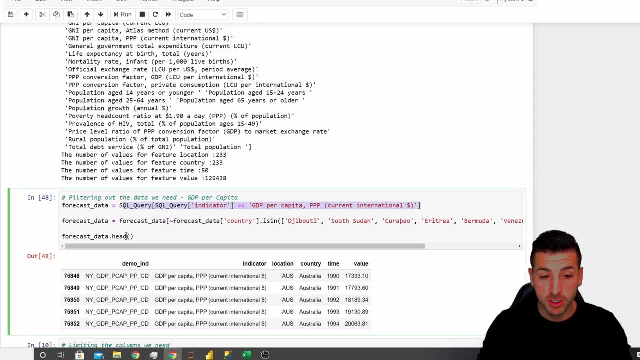 thing I want to forecast going forward. Additionally, I also exclude a few countries from our data set. The reason I'm excluding them is because they have some problematic data that I have identified later on on this analysis, but just for ease of this tutorial, I'm just deleting them from here. So 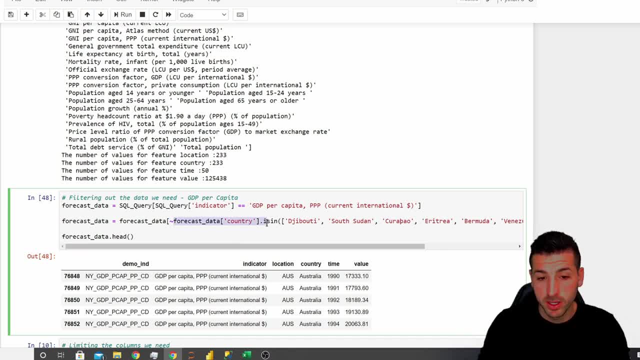 the way to delete them is actually run the same code where you say dot e scene. but if you add this symbol at the beginning of your data frame just before you run, the e scene is actually going to exclude them, And then I'm passing it back into this data set. So if we run this, we get 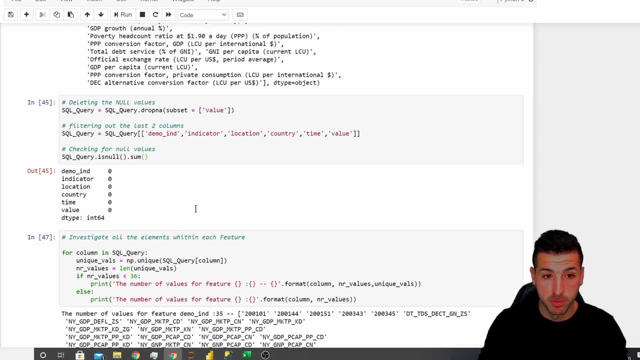 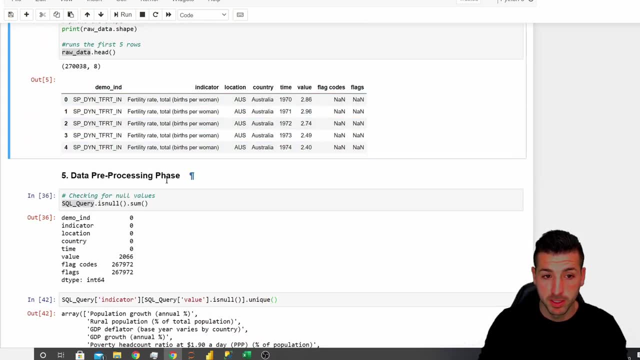 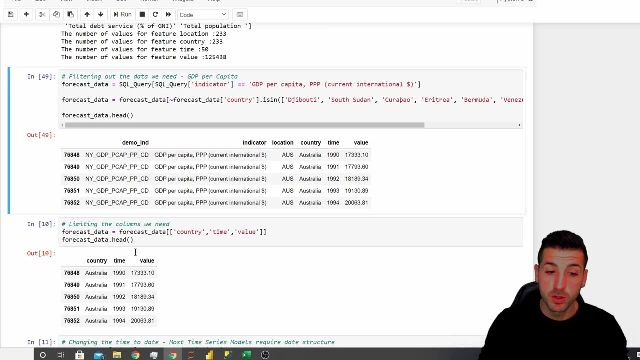 the same, the same columns as before. we have above here, but now we only have one indicator. So in indicators- before we had multiple indicators, now we only have indicators equals to GDP per capita. The next thing we want to do is to limit the data to the columns we need. So we only need country. 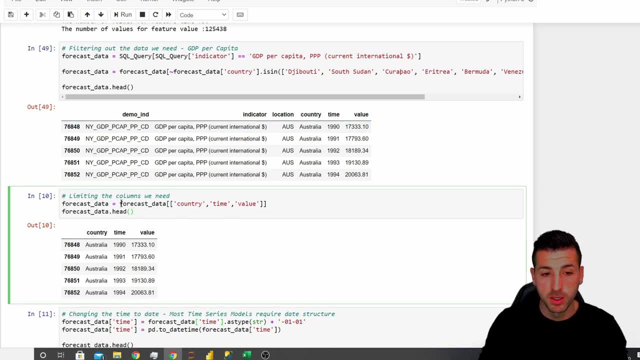 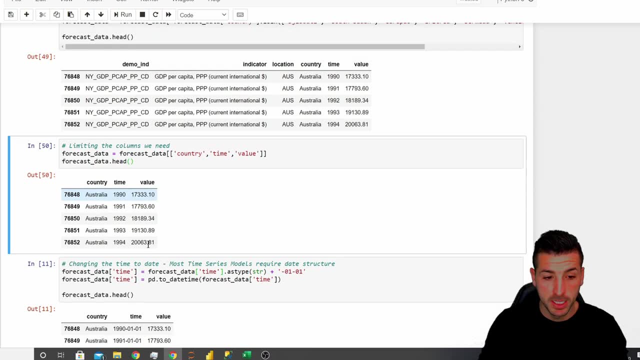 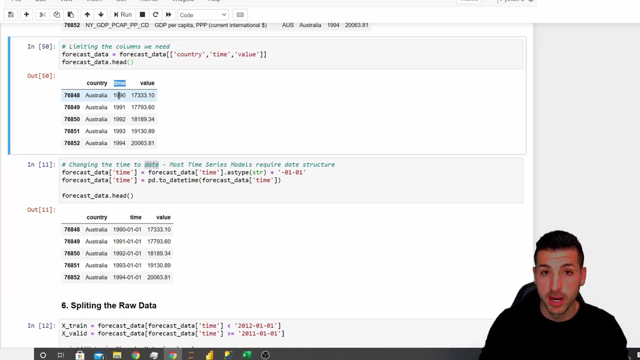 which is this one time and value. So what I'm doing is that I am passing these three columns back into our data frame, So you can see we limited the data. The next thing we want to do is to change the time to date. So change this column to be an actual date, as most time series models. 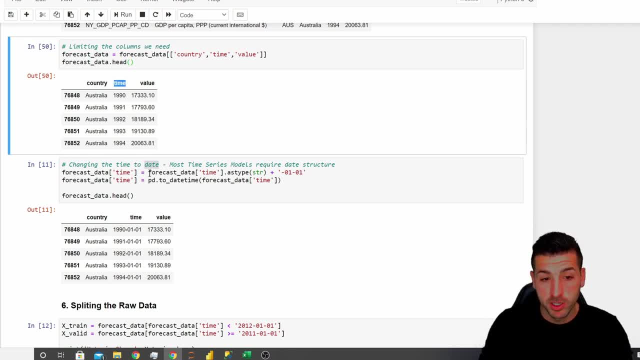 require a date structure To do this. I'm just taking the time, I'm making it a string and then I'm adding the dot zero one and then the dot zero one, as you can see it over here, And then I'm passing this. so now it's a string, remember, and I'm passing it into a PD- dot two- date time- and then 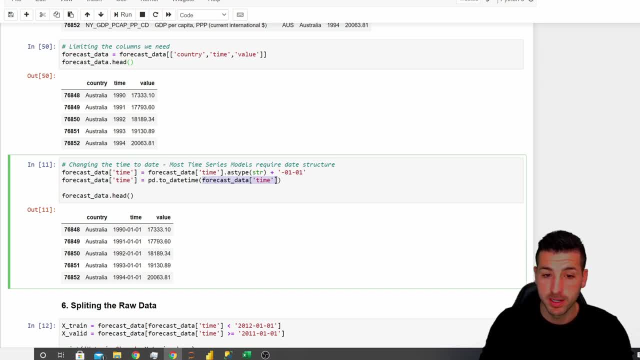 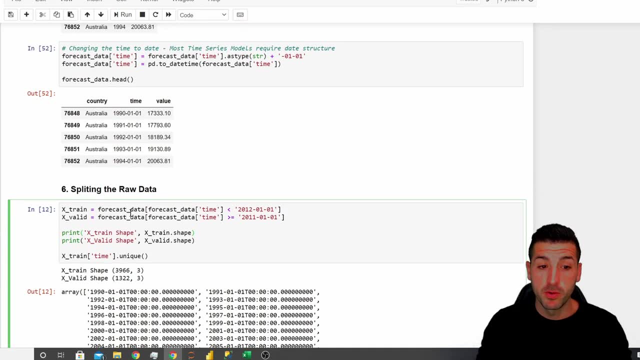 I'm passing into two day time before cast time, So now this time is actually a day and it's actually a day time. The next step now is to split our raw data into X train and X valid. Our X train is going to have all the data before 2012 and our X valid, which we're going to use for evaluation and 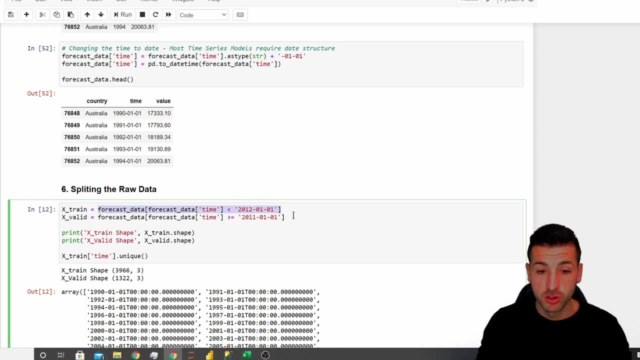 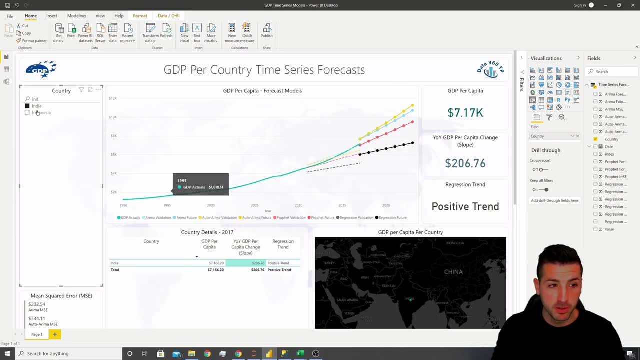 here. it's going to have data after 2011.. So just to visualize this, because we do have the output, if I go over here, imagine that I am splitting. so this is just India, but I'm doing this for all countries. I am splitting all these GDP up until here. so imagine I'm putting a line here. 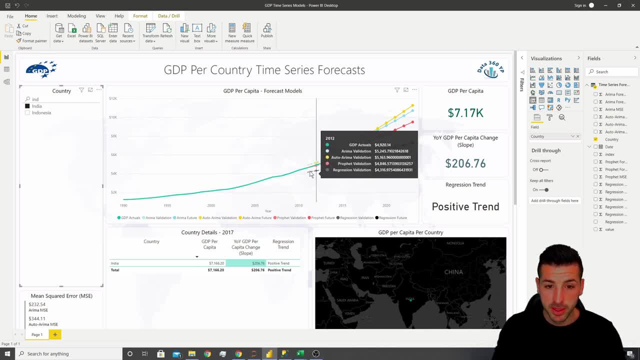 and then I'm selecting all of these for training data and then, from here- 2011, all the way to 2017- the green line I'm going to use for a validation data set, Which is exactly what I'm doing with this code over here, and if we print the two shapes, we can 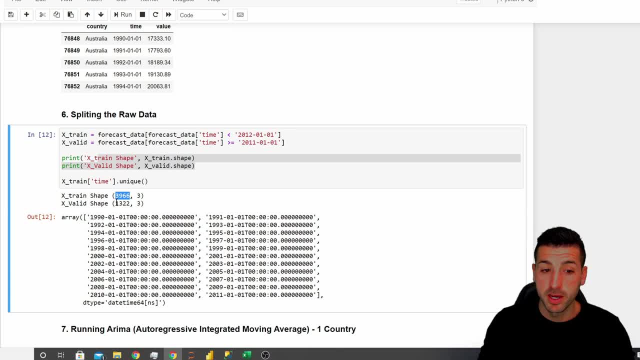 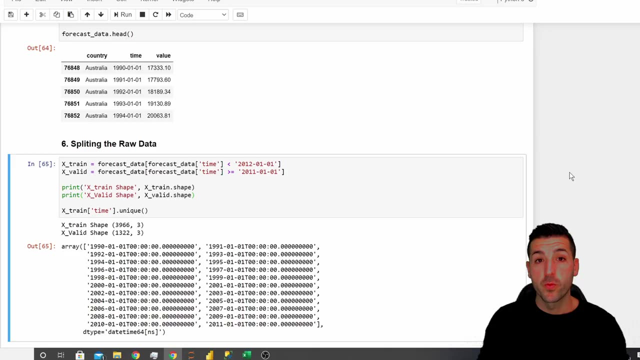 see that our training has about 3966 observations and our validation data set has about 1322 observations, and both of them have three columns and the columns are country, time and value Right. moving on, we are going to run Arima, which is auto regressive integrated moving average. 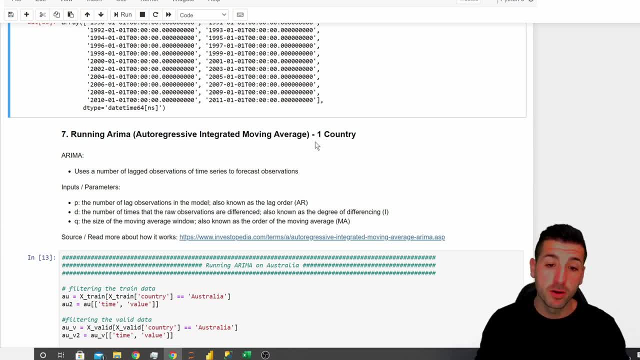 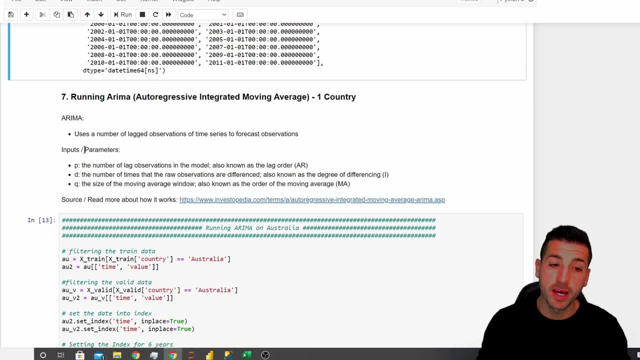 time series forecasting model and we are only going to run this on one country for now. just to simplify things, A few notes on Arima now. Arima uses a number of lag observations of time series to forecast future observations and it takes as inputs and parameters the B, which is the number. 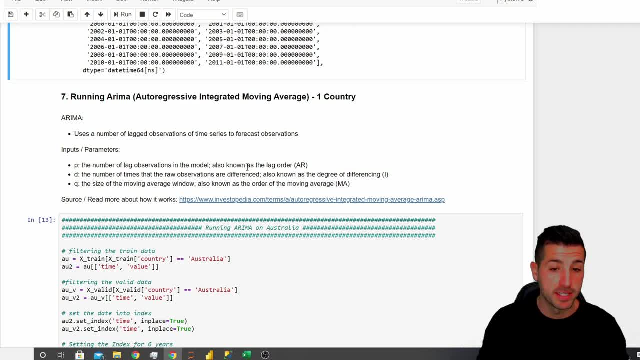 of lag observations in the model which is also known as the lag order, and this is the AR. so the number of lag observations is very impressive: the D, which is the degree of difference, which is the integrated, and the Q, which is the size of the moving average window, which stands for MA, which 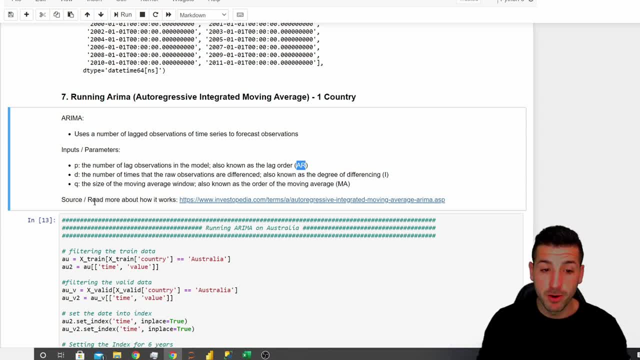 is the moving average. If you want to learn more about Arima, you can follow this link and read more about the math of Arima and how everything is calculated. I'm not going to get into it, just because this tutorial is more focused on applying it rather than using it. 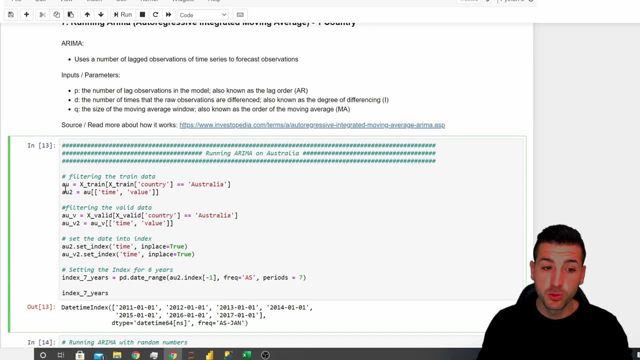 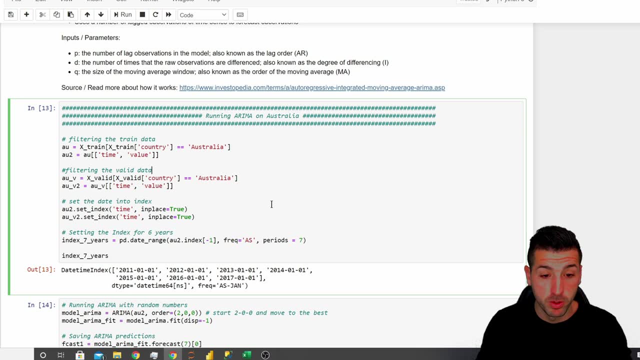 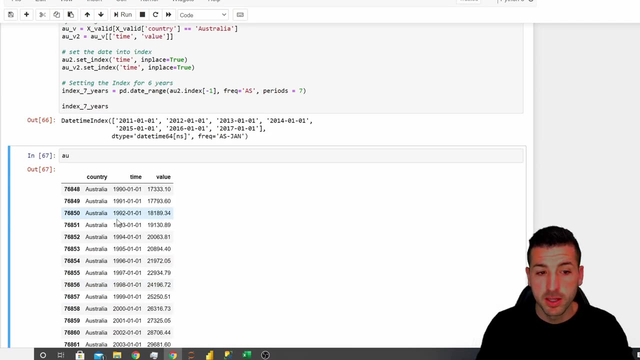 explaining it Right. so the first thing I want to do is to create two new subsets of data that have data only for one country, and I'm going to use Australia as an example. So I create this AU. so if I copy this quickly, I run it and paste it, you can see that we only have data for Australia. 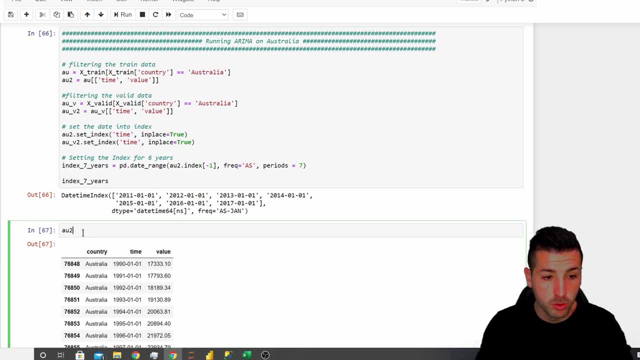 in this data frame and I also create the AU2, which is just the time and the value for this data frame. I repeat the same process for our validation data set, because I'm going to use these two to validate our results. Then what I do over here is that I set the time into an index, as you can see. time. 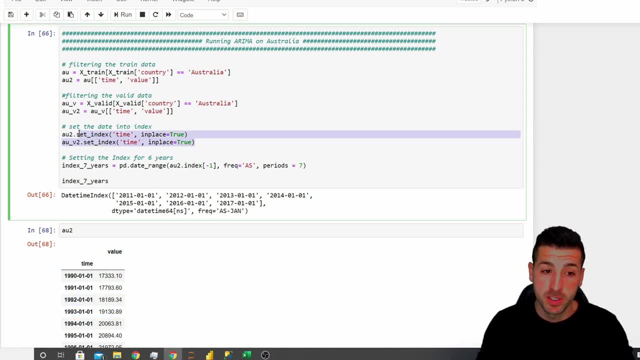 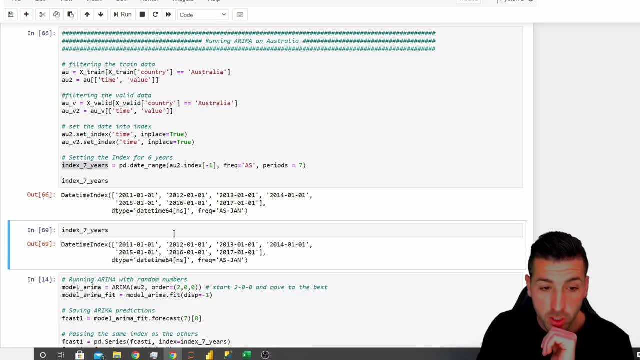 is now an index. you have to do this to run a time series models and the last thing I do is that I create an index for 7 years going forward. So, as you can see over here, the index I'm creating, it's range from the AU2 index minus one, so it takes this AU2 index minus one. it. 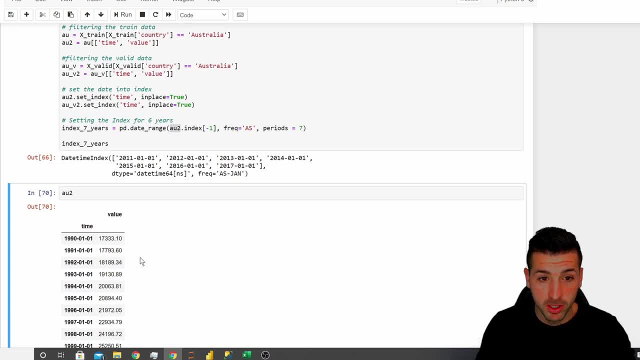 means that it's going to take this last value and it's going to use frequency as AS, which is an annual frequency, and it's going to use seven periods. so it starts from here and it adds six more years, as you can see, from 2011, all the 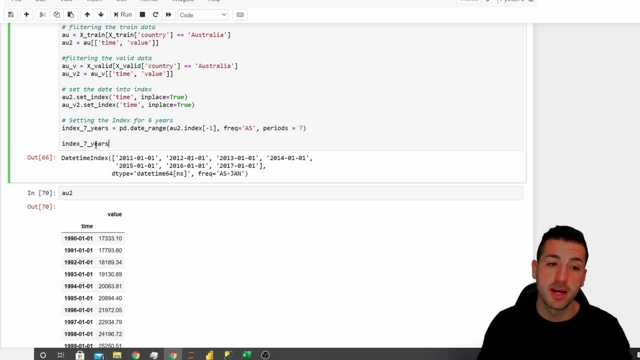 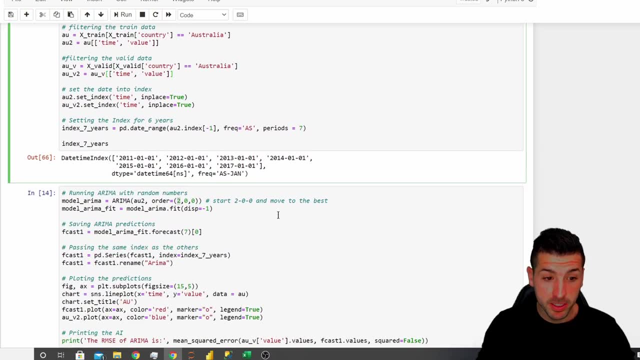 way to 2017. the reason I've done this is that I'm going to use this index to make predictions, to to use it as a forecasting input, right? the next step now is to run Arima with just some random numbers, so I call the model Arima. 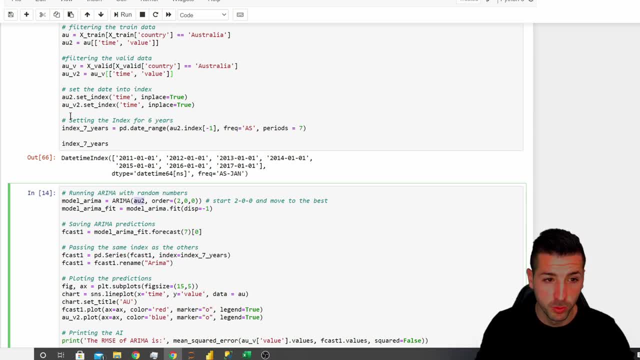 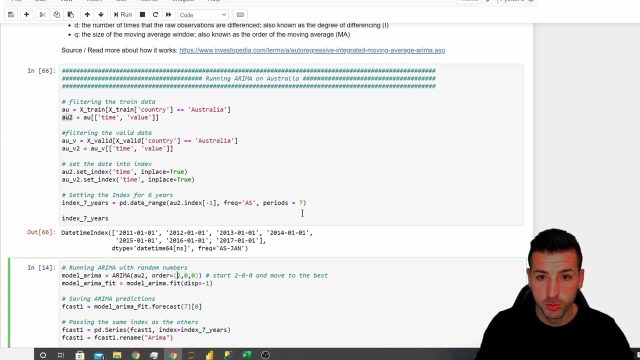 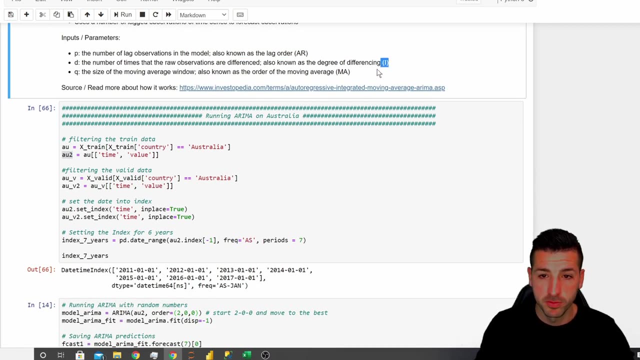 and then into the model I feed the AU2, which is the AU2 created over here, I give a random order of two, zero, zero. so two is actually the auto regressive. so from here the zero is the degree of difference, so the zero is my I. and then 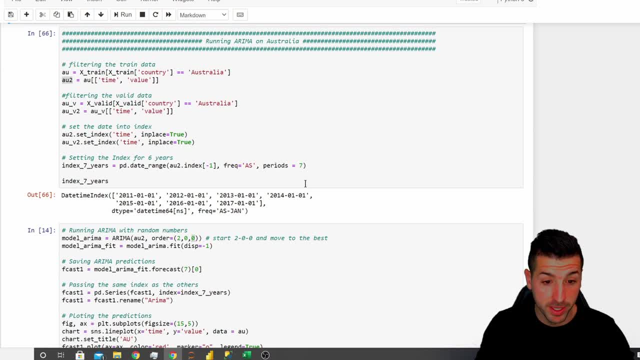 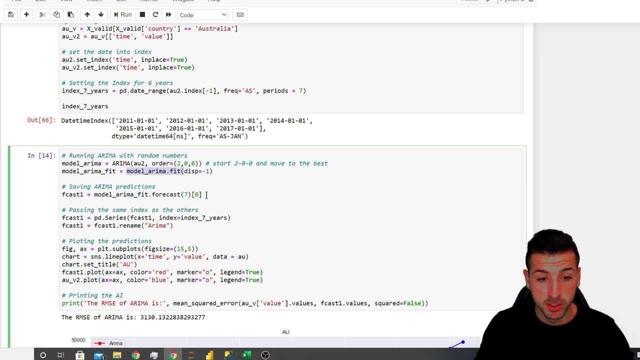 the last zero is the moving average we have from here, and then I feed my model with discrepancy equals minus one. then I create some predictions. so I call my model model Arima, underscore, feed, dot forecast. I want to forecast seven data points and I want to take the first row. then I'm passing the. 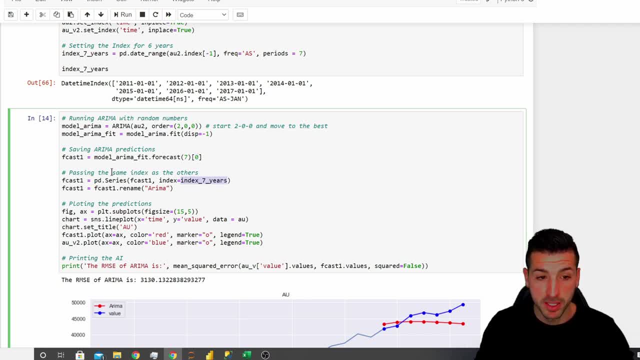 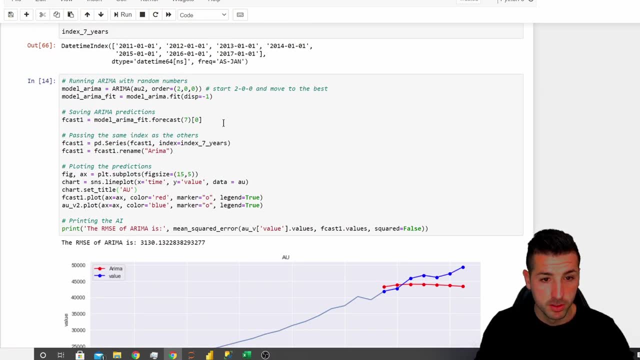 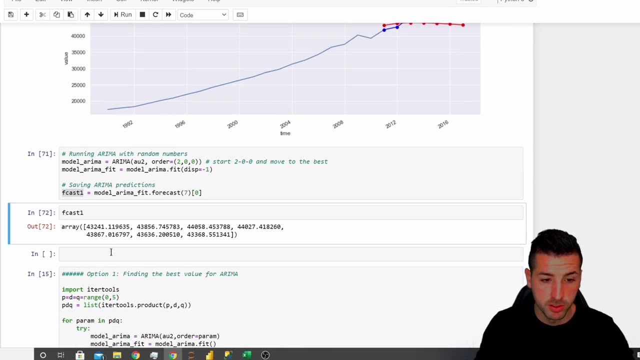 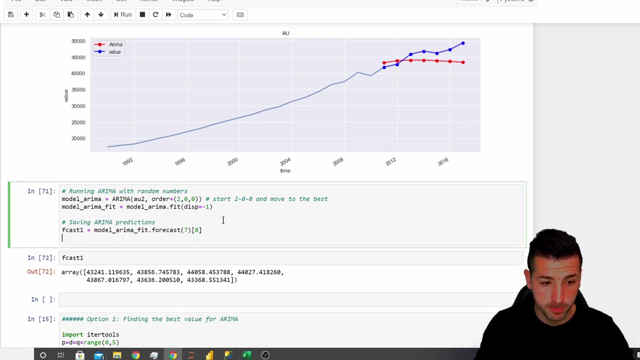 same index as the index I've created into my forecast. so just to run it bit by bit to show you, let me just create this: if I copy this and run it. so my forecast- now I copy my forecast- is just seven numbers without an index, and then if I run these it means that I'm gonna pass. 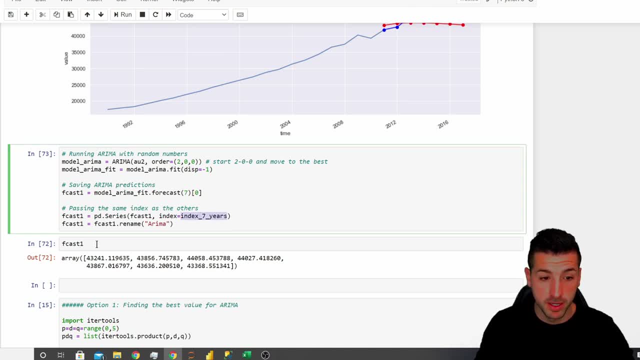 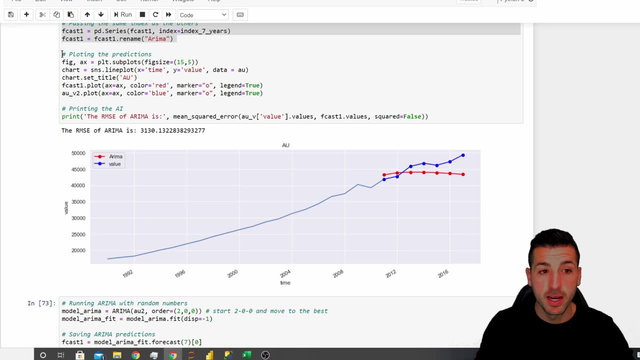 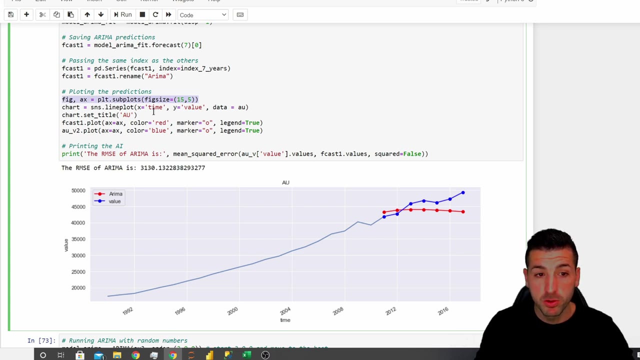 this index I've created of those seven days forecast. so if I run this now, you can see there is an index on my forecast. and the last thing I do here is that I plot my predictions. so I initialize an empty plot with this line of code, then I pass a line plot which is this blue line over here: x- I'm using time, y- I'm using value and. 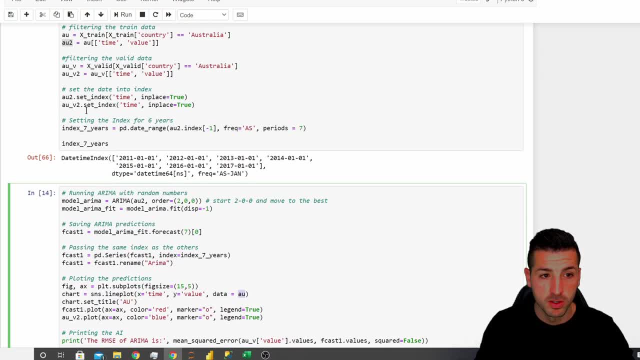 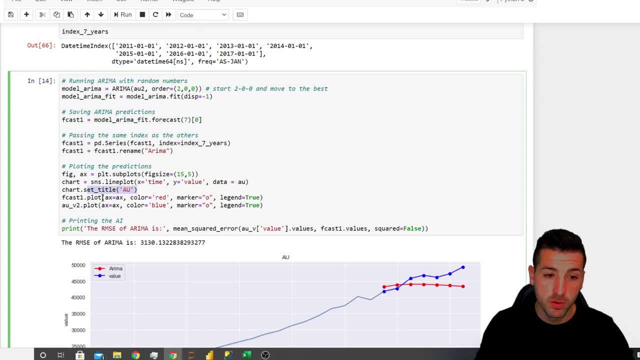 data. I'm using the au, which is the first one, not the indexed one, and then I'm setting the title into au and then I'm creating two additional plots, which is two additional lines. the first one is the red one, which is my au color. sorry, yeah, the red one is the forecast, because I'm 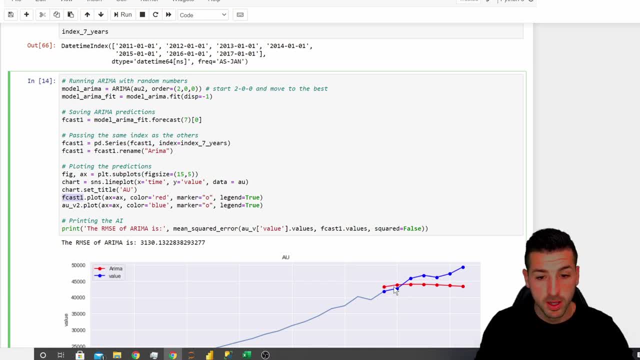 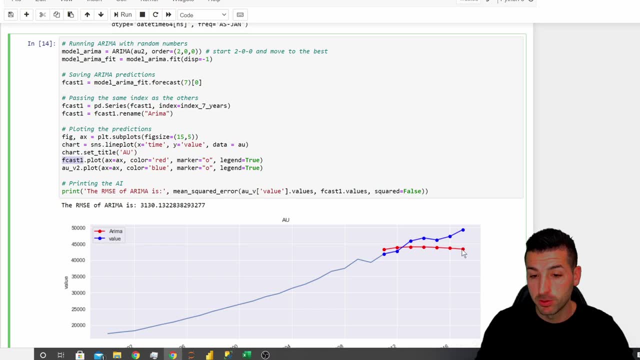 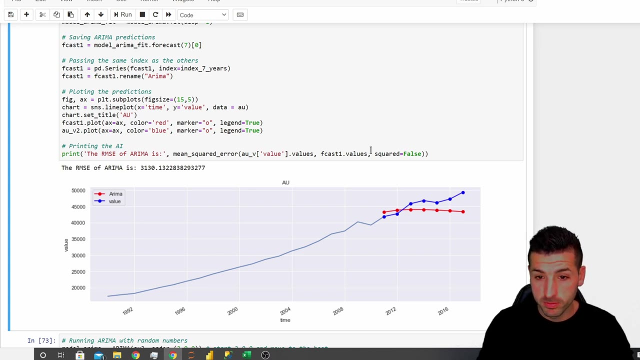 the forecast one dot plot. so red is the forecast and blue is the actuals. so, as you can see, we haven't done a very good job, as our prediction is going plateau while the actuals is still going up and the last thing we print is the root mean square error. it's actually the mean square error. 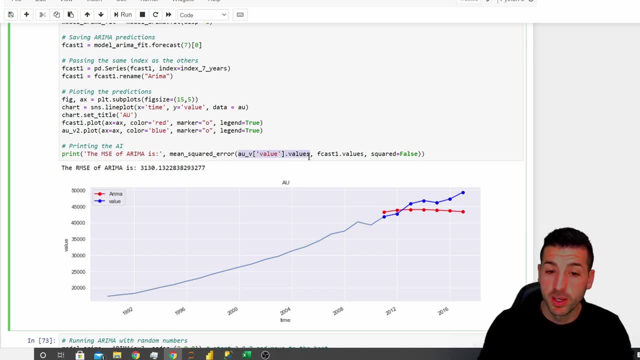 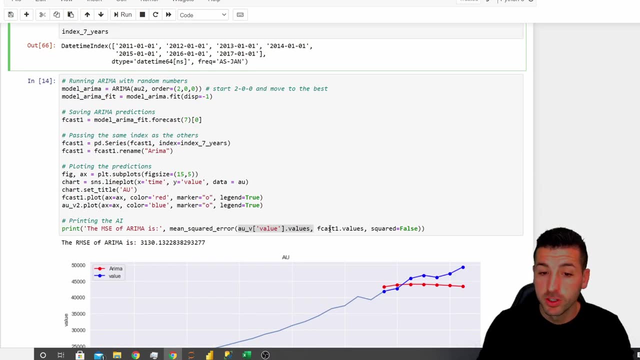 not the root mean square error which takes us inputs the actuals, so the- this is the- comes from valid, from the validation over here- and then the values then takes, it compares them with the forecast values, it calculates the difference, it takes the mean and then it squares the mean. but I'm not squaring the mean, it's just the mean. now. 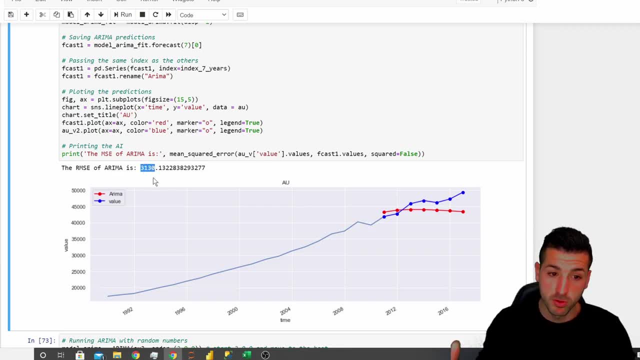 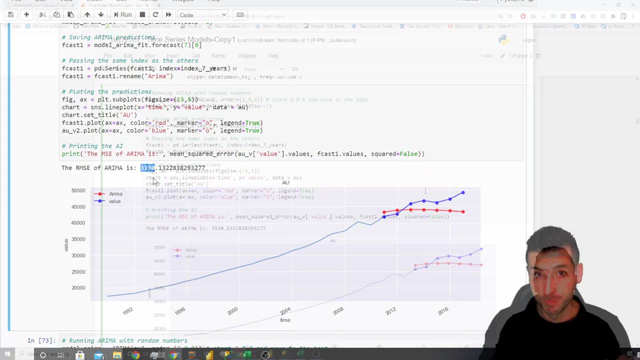 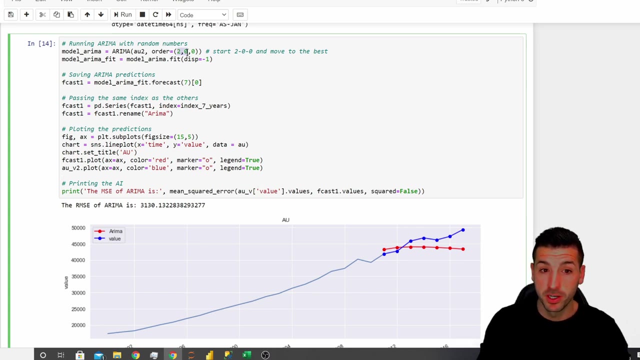 so what this is telling us is that our predictions from our current model are off by three thousand one hundred and thirty dollars on average. the next thing we have to do now is to try to improve our model, and to do this, we have to try multiple different combinations, in this order over here: 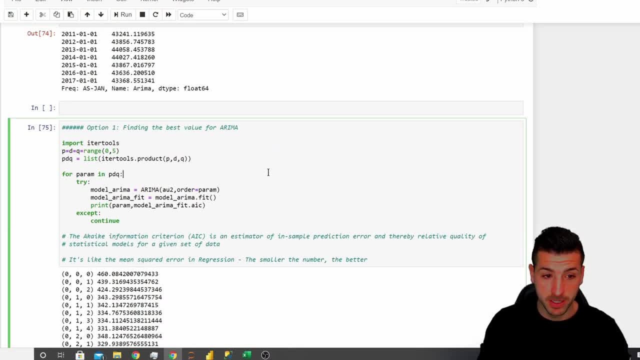 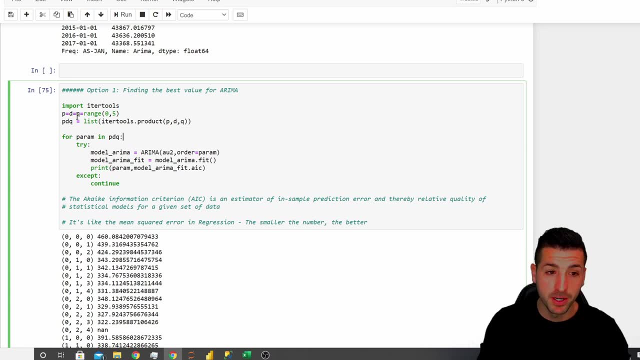 one way of doing it is this piece of code I have down here. what I've done down here is that I've created a range of p, d and q from zero to five, and then I get I pass the dot product of this range, zero to five, into a list. so just to let you know what this is. 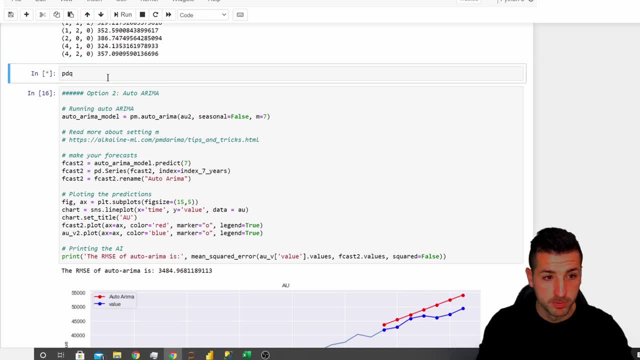 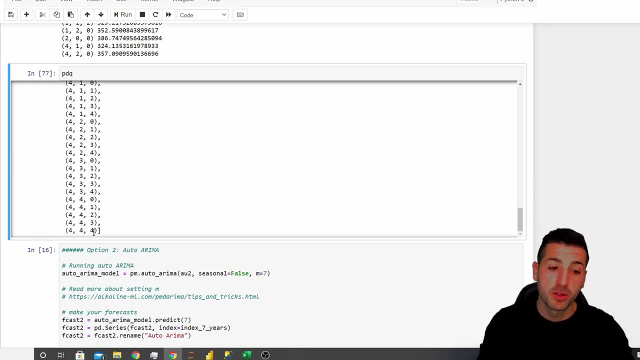 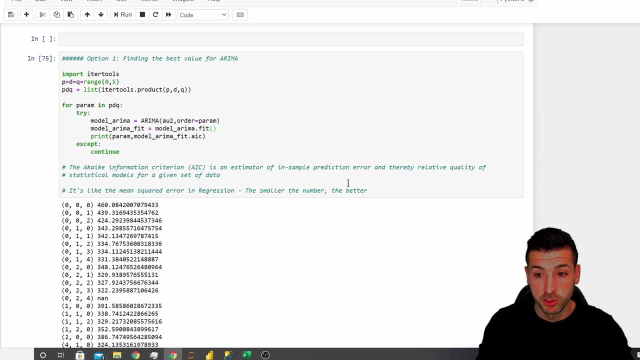 if I copy it and paste it down. here is all possible combinations from zero to five. and see, I keep scrolling, it's not actually five because it starts five from zero, but it's five different numbers and all of their possible combinations for the dot product. what I do here I say for parameter in pdq, I try to feed a rima again on the same data set. 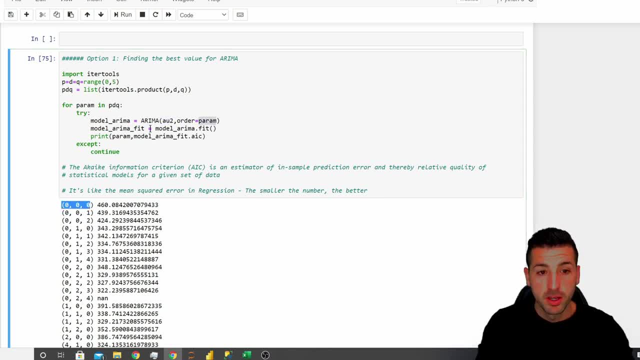 and passing the first order which is going to be this order, then I fit the model and then I call the aic. so the aic is the archaic information criterion, which is an estimator of ensemble predingsure error and thereby a relative quality of statistical models for a given data set. 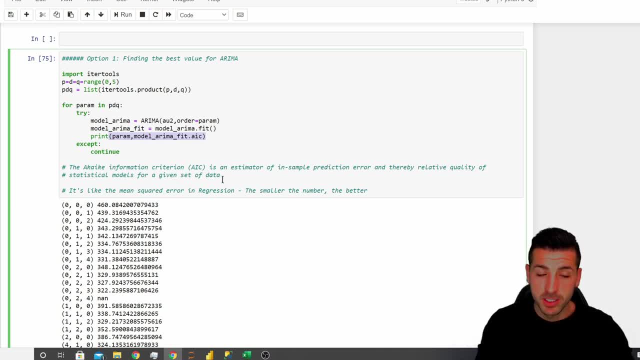 so what it means is just a metric that evaluates how good your feed is, and it works like the mean square error, so the smaller the number, the better. it is what this code did. now, if I run it, it goes through every possible combination and it prints this aic, and what we have to do now is to choose the combination with the minimum a. 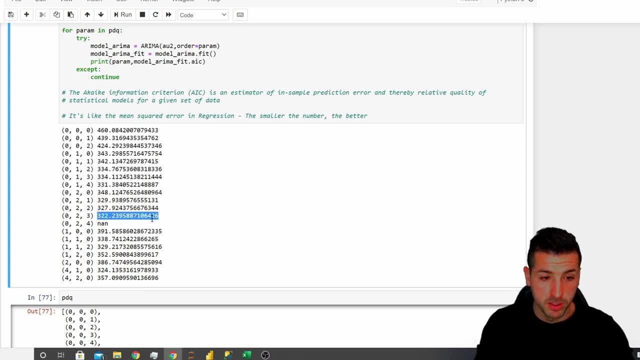 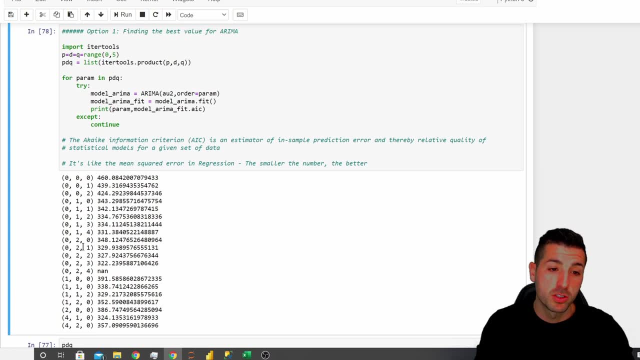 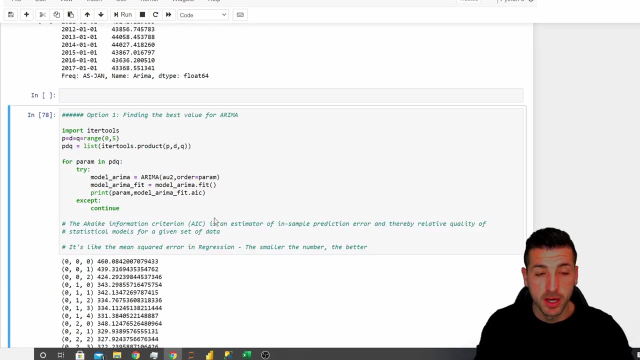 I see which is this one: 0, 2 and 3, as you can see, is the minimum. You can also see that we don't have all possible combinations, and this is because Arima is not going to work on all possible combinations. So, for example, 4 4 4 is not here and if I put 4 4, 4 at the top, it's going to throw me. 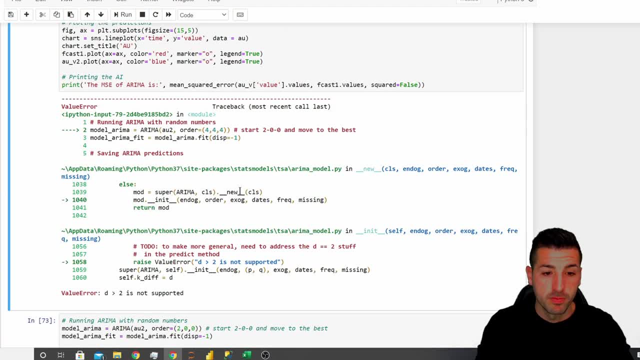 an error. There you go, So you can see, d more than 2 is not supported based on the data set we currently have. So what we need to do now is to try this combination: the 0, 2, 3.. As you can see, 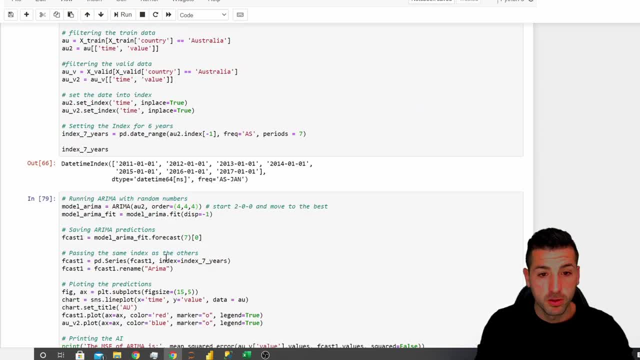 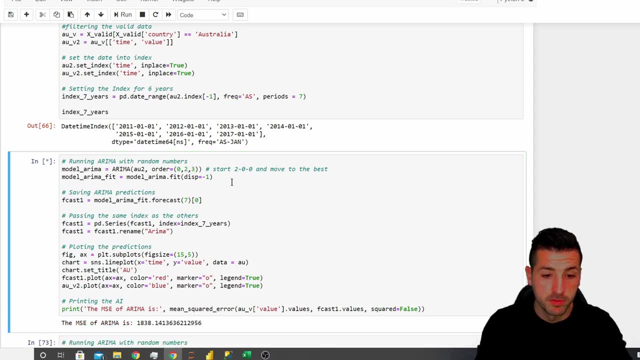 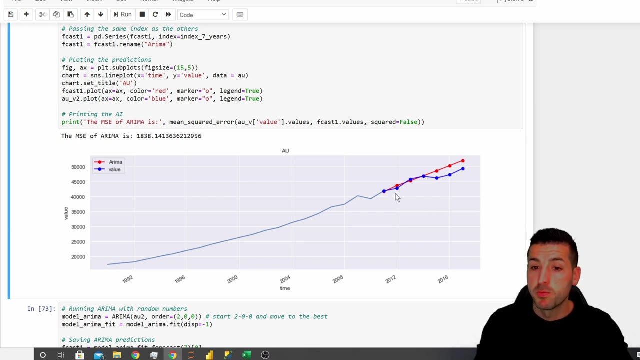 it gives us the lowest value. So if I go at the top and I do 0, 2 and then 3 and if I run this, you can see we have a much lower mean square error and you can see our prediction is much closer to the actuals. 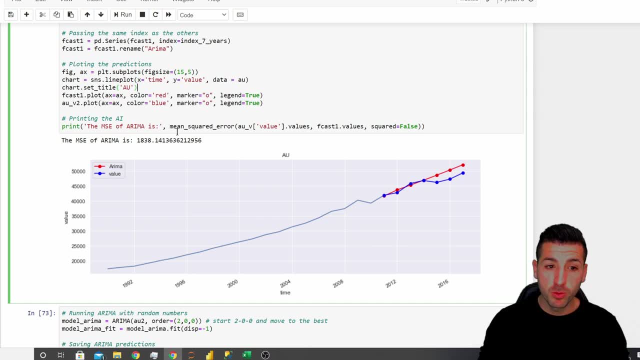 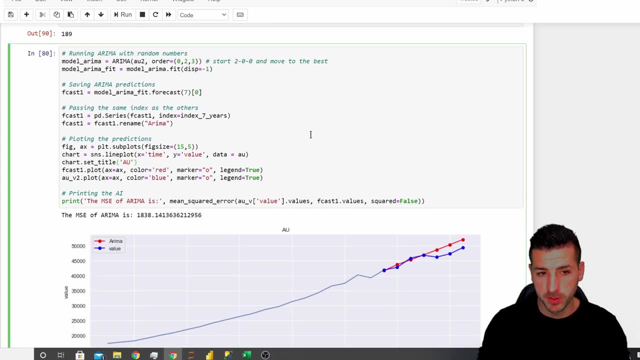 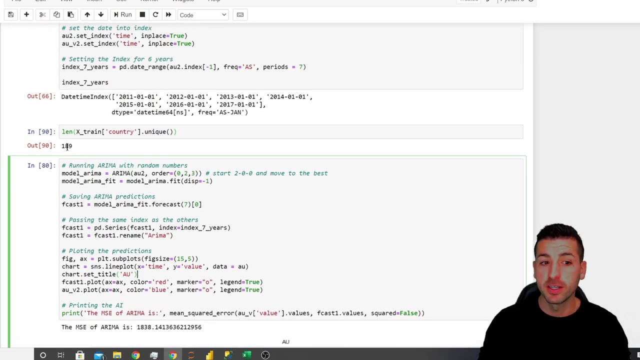 The challenge now with this method is that we have only done one country, which is Australia, and different countries are going to have different optimal parameters. So imagine doing these, repeating the same process as we've done here, 189 times, which is the number of countries we have. It's not very effective. 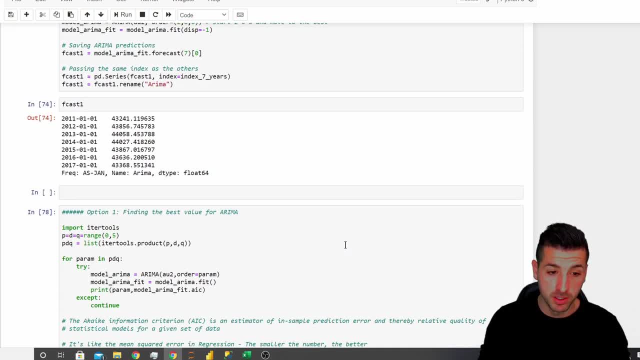 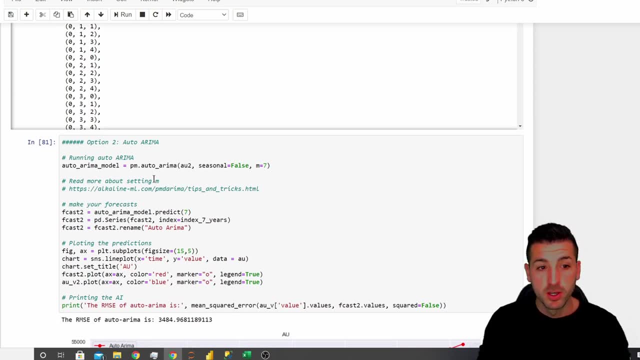 So this is where auto Arima comes into place. If I scroll down, here is the second option where we have the auto Arima model. So to run auto Arima is very similar with the Arima. So you just call the model, you fit the same data in, you say if there is seasonality or not In our case, because 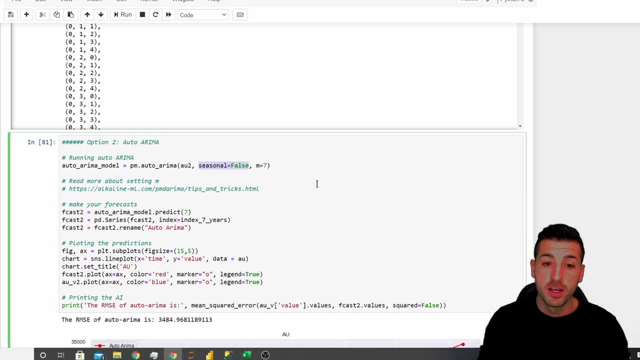 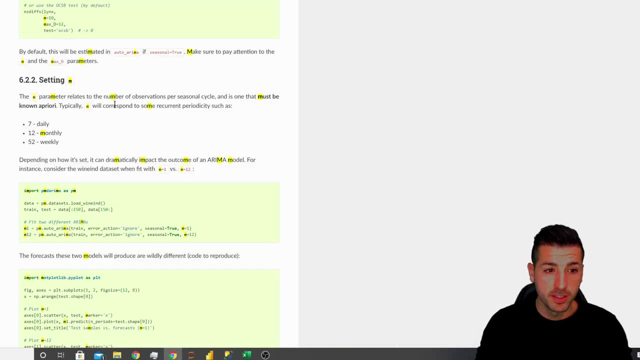 it's GDP per capita. there is no seasonality. and then you have to set the m. Now the m is a bit challenging because if you read about what is the m, the m parameter relates to the number of observations per seasonal cycle, and that is one that must be known from before. So, because we 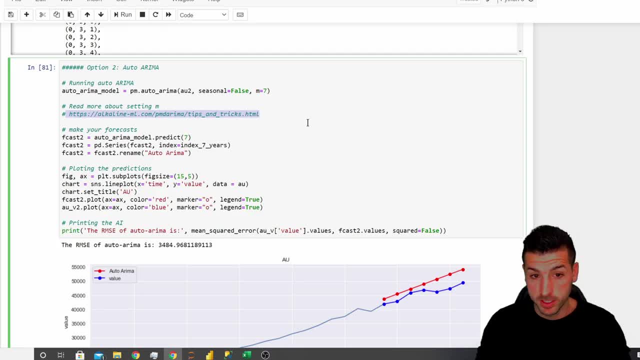 don't have any seasonal cycles for GDP as far as I know. I'm going to try with 7, and I'm also going to try with 10 and 15.. Remember, we use years, So if I run this with 7, by the way, everything else is. 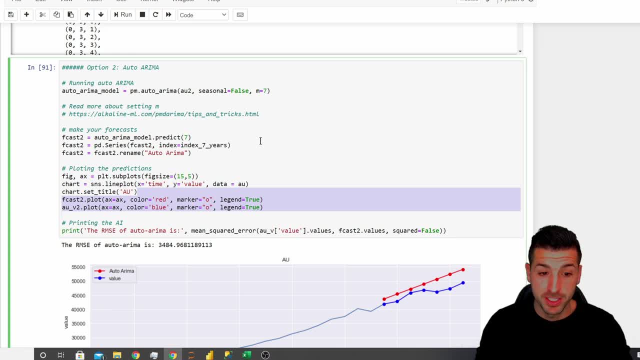 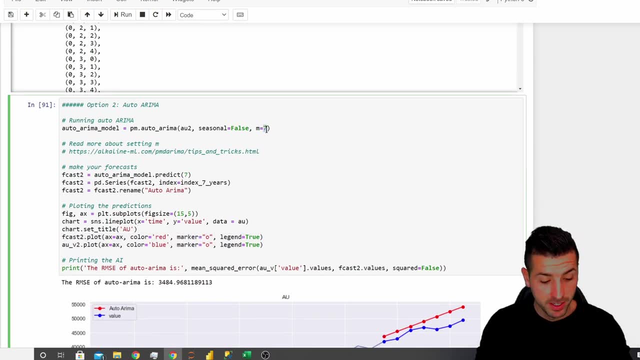 exactly the same as before, The previous code which we have just explained. you can see that 7 is not giving us a better model than the one we have identified. Then if we try 5, maybe so 5 still is not as good. If we try 10. 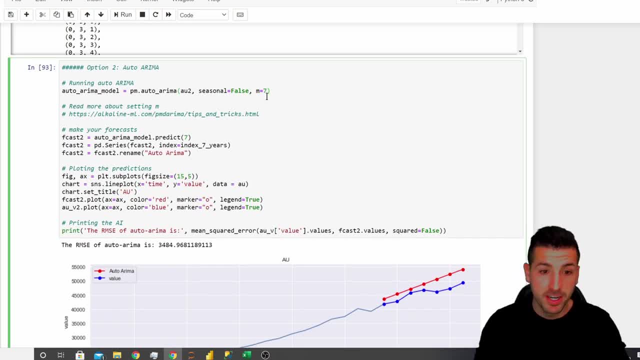 still not the best, So I'm just going to leave it at 7.. And my main point here- why I have both Arima and auto Arima- is that you cannot be certain that auto Arima and auto Arima are the same. auto arima is going to pick up the best parameters. my conclusion is that you have to run some auto. 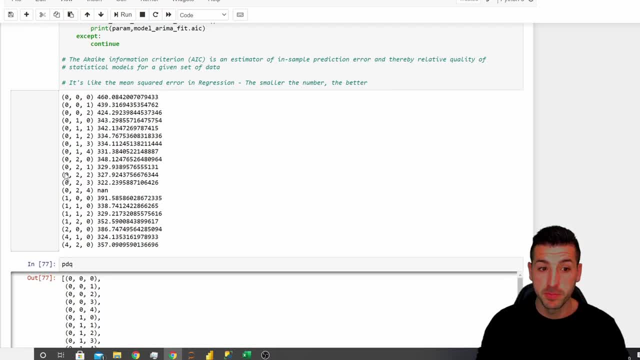 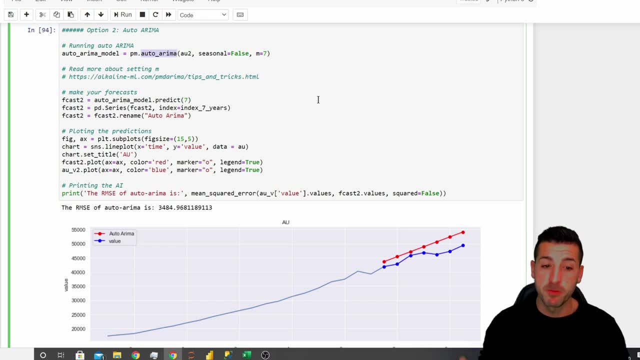 ones. so when i say auto, i mean the manual ones- find the best parameters and at the same time run the auto arima, just to compare the two together, which is something i'm going to show you later on when we combine all the countries and the models together. right data friends, i'm 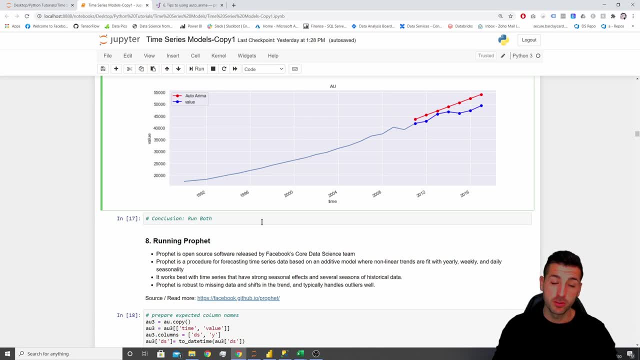 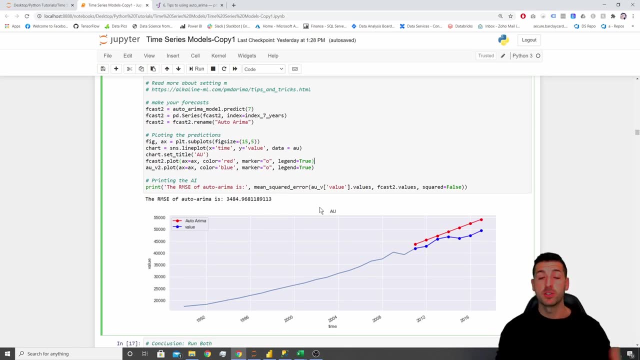 going to stop this tutorial here and finish the rest of this series in the next video. so i hope you've enjoyed this video and you've gained enough value out of this video. if you feel like you did, please click the like button. subscribe to my channel. enable notifications for my future. 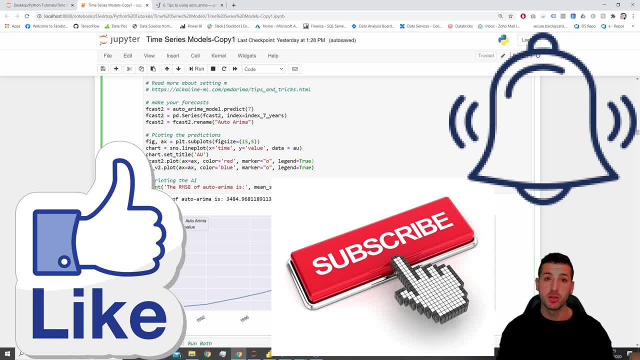 videos and if you have any questions, please let me know in the comments below. otherwise, thank you very much for watching this and i'm going to see you in the next video.